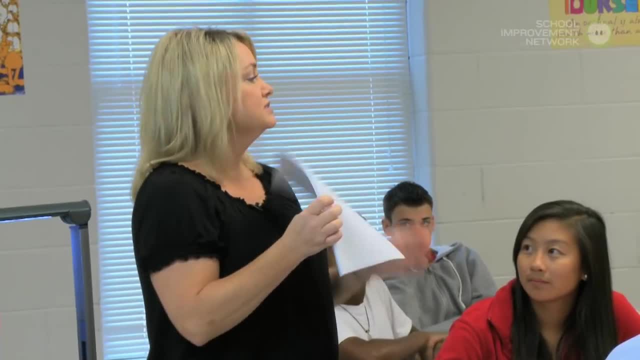 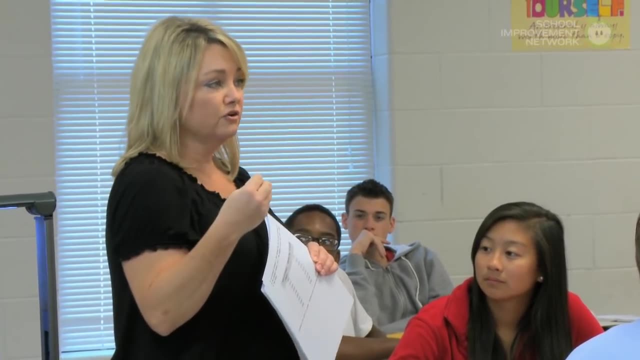 1900 to 1996,. okay, Once I give this to you, I want you to think for a few minutes all by yourself, some private think time. okay, Think about how you're going to graph this. okay, Think about. 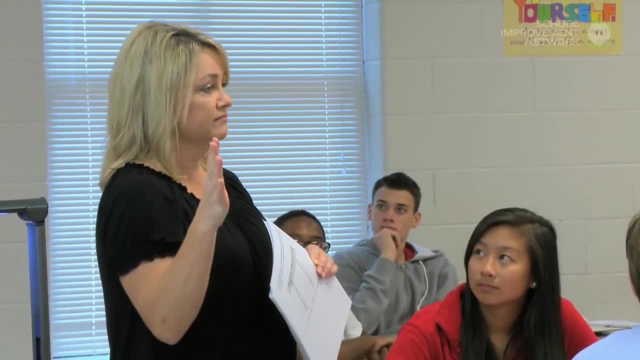 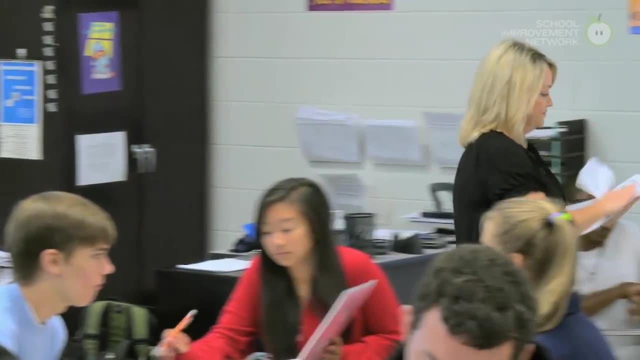 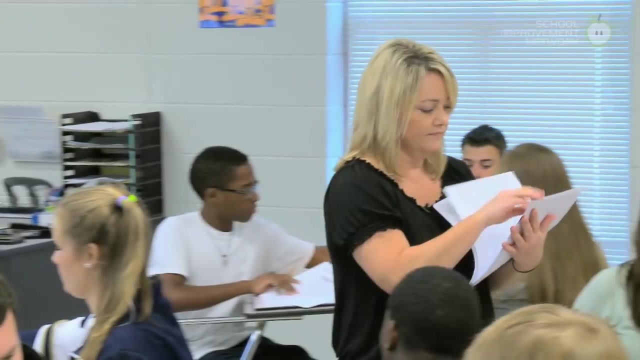 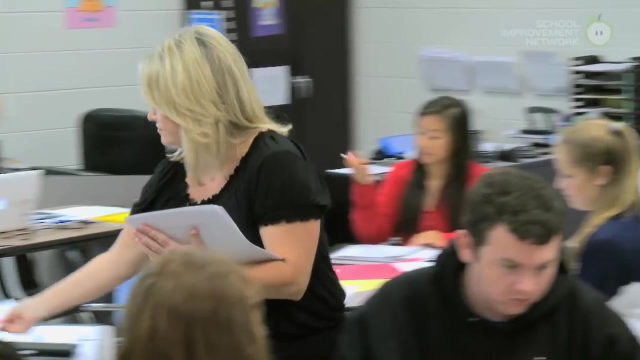 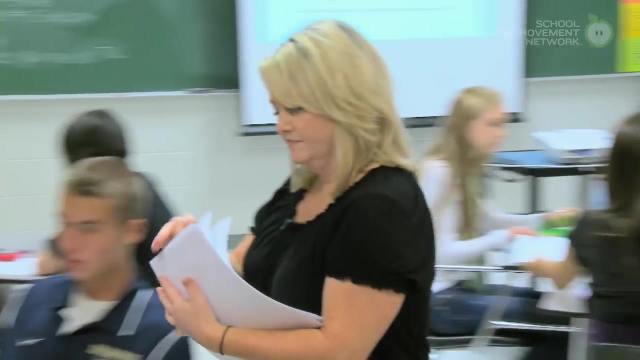 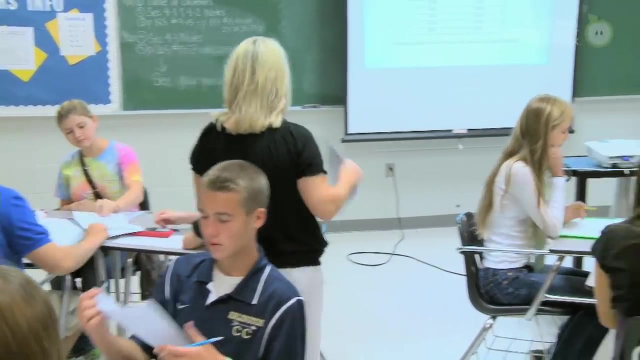 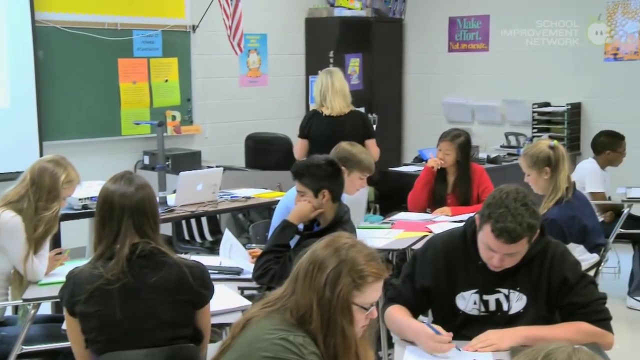 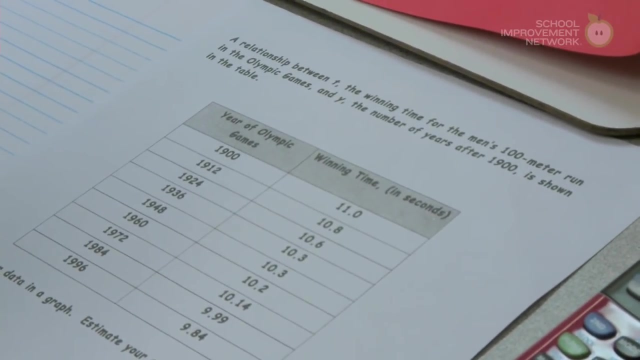 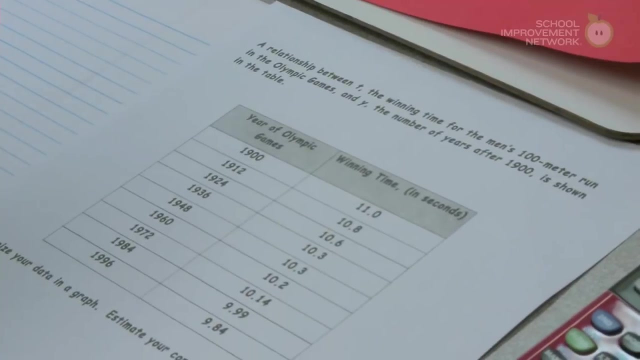 your X and Y axis, Think about your labels, Think about everything, okay, And then, after you have some private think time, we're going to do this in your groups. Okay, Thank you, You're welcome. There you go. Okay, talk a little within your group and decide how you want to set up your graph, how you want to. 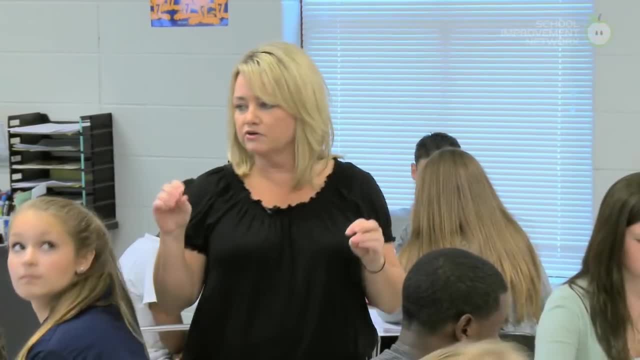 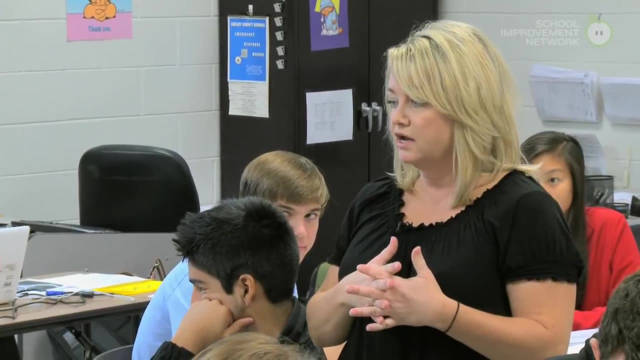 set up your scatter plot and then, on the yellow piece of paper that's on your table, I want you to graph the scatter plot for me. After you've graphed your scatter plot, I want your group to come up with the best correlation coefficient you can get. Estimate what you. 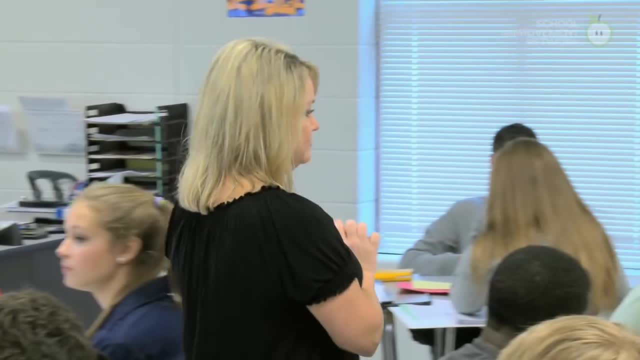 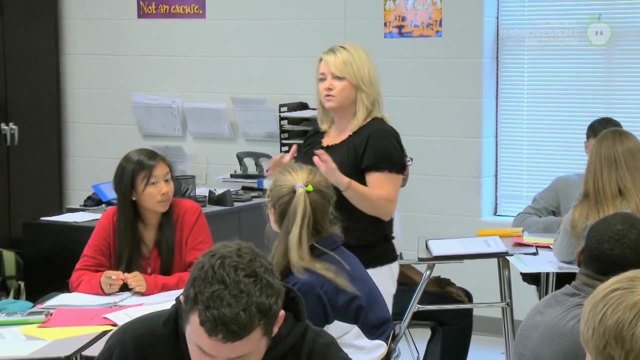 think the correlation coefficient's going to be okay And let's go ahead and round that to the let's do the thousandths place, because we want to have a winning group, because you might get a little surprise if you're the winning group. okay. 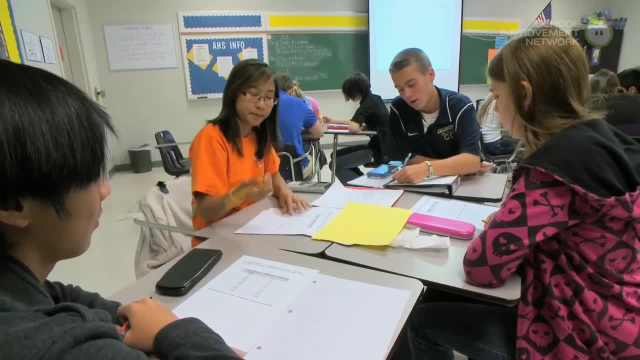 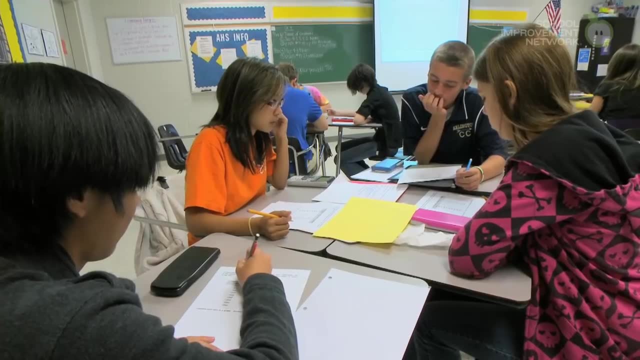 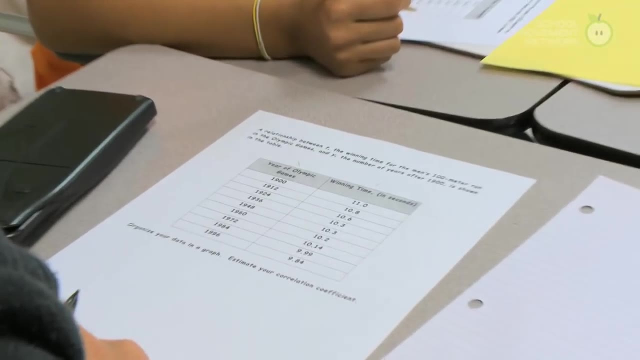 Okay, All right, I'm going to put the year of the Olympic Games as X, and then, since that's an independent variable, I'm going to put Y as the winning time. Then, yes, What should we go by? What We're going to go by the 1900s. 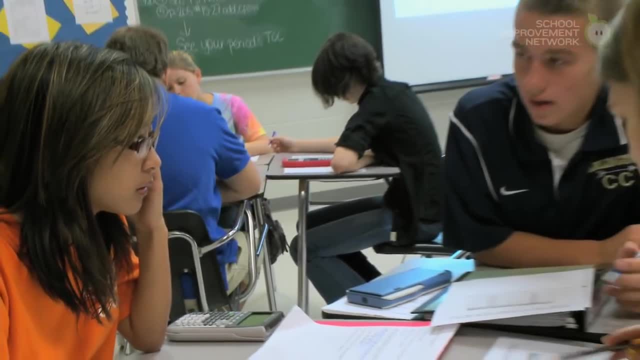 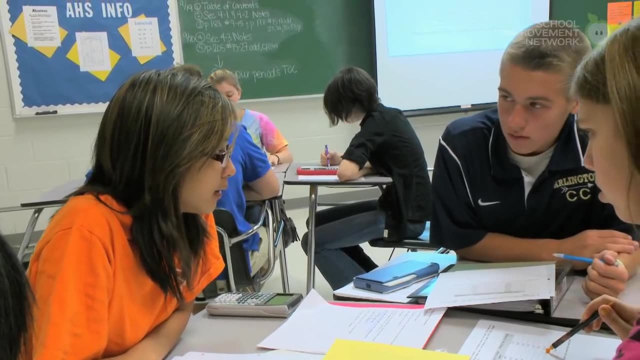 That's our scale. It's going to be way easier if we go by 1900s, like, instead of doing what we did yesterday. I'm talking about our scale, though, like, because on the scale, yeah, What about it? 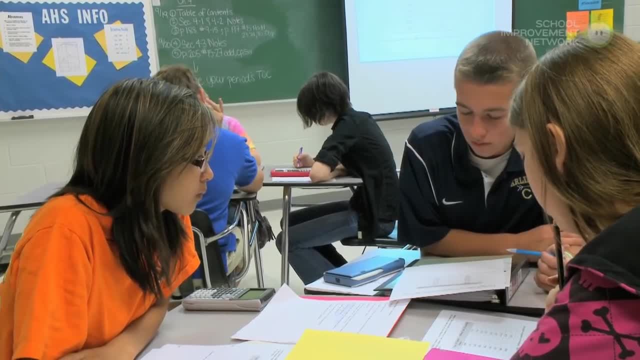 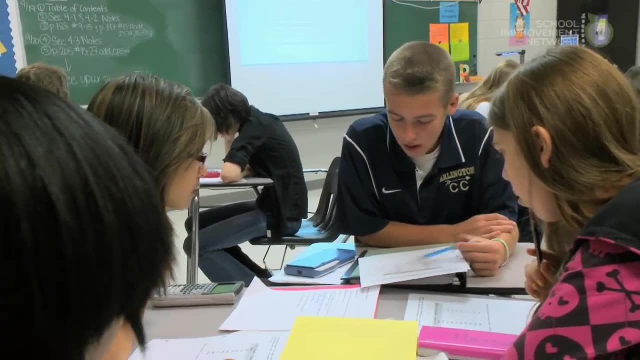 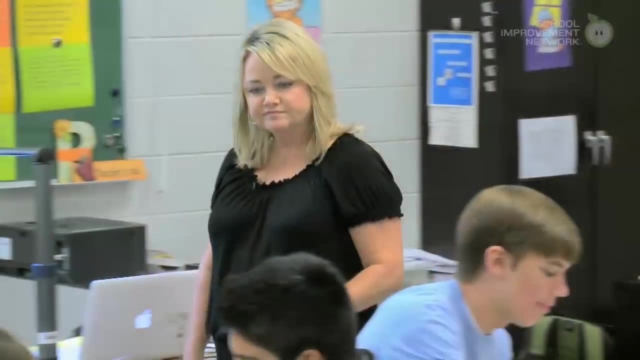 I would do like 9.8 or 9.2.. For this one we should easily go by 12 or 900.. This one probably, yeah, by .2s or something Maybe .4s. Can we do like exactly the year, like that? 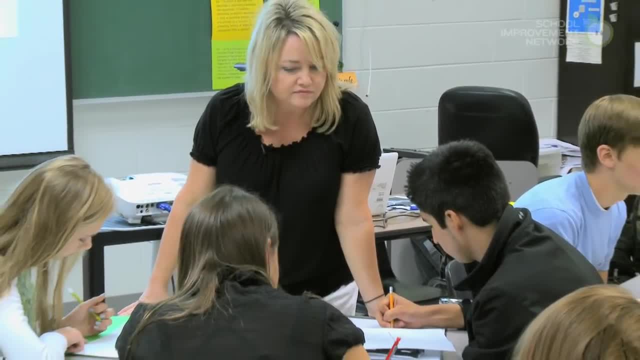 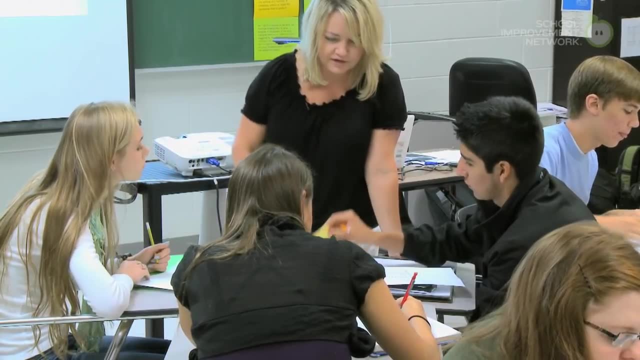 Sure, Mm-hmm, If that's what your group wants, Just make sure you label And one of you, I want one of you to do it on the yellow. okay, It's not starting at zero. Perfect, What's that called? 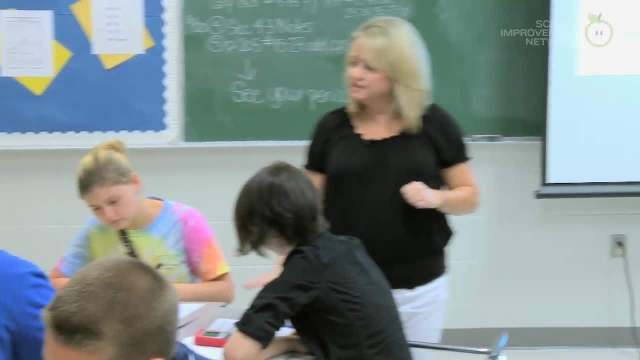 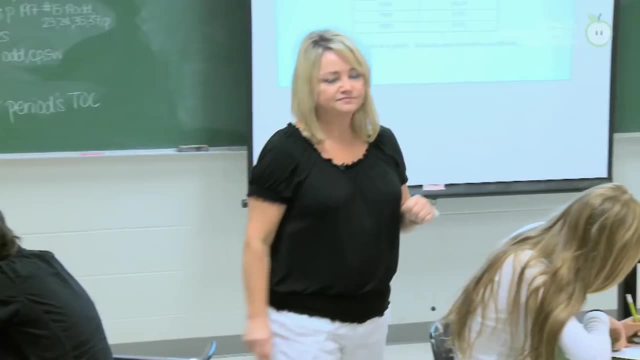 The break, The break. It's a good one for technical The break squiggly thing. I know what you meant, right, 9.6.. Good job, Good job. What scale did y'all decide on? Ten, 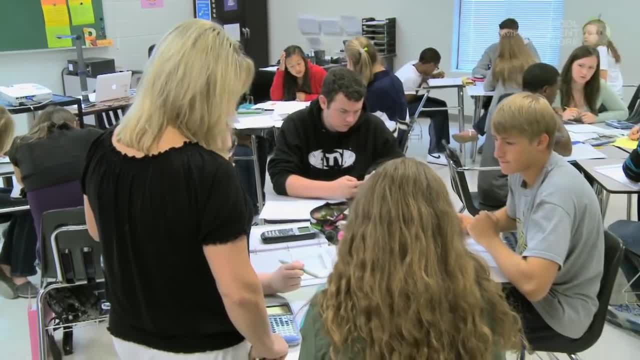 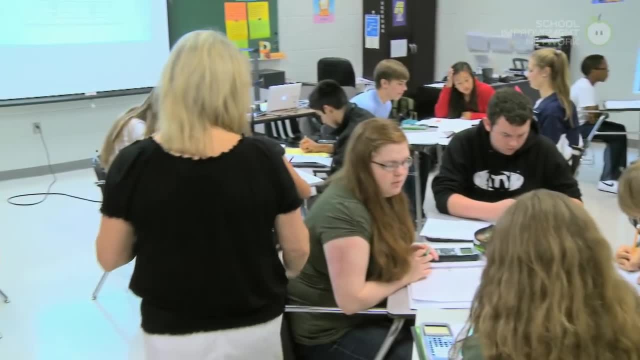 Yours at zero. Awesome, And you're going to do tenths? Okay, We're going to do a break and start at 9.8.. Perfect, Sounds good, Christian, we're going to do the calculator later. okay, Help them with that graph. 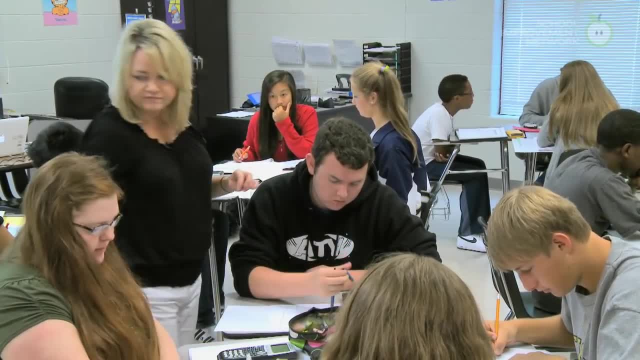 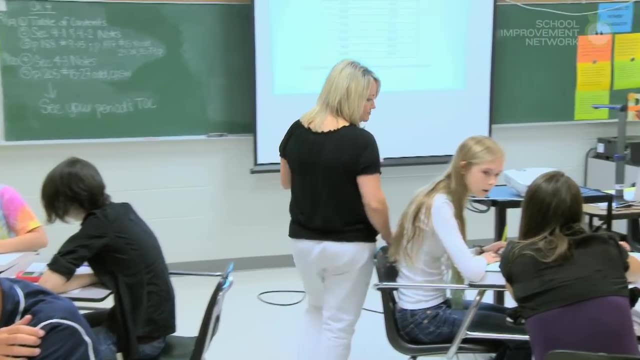 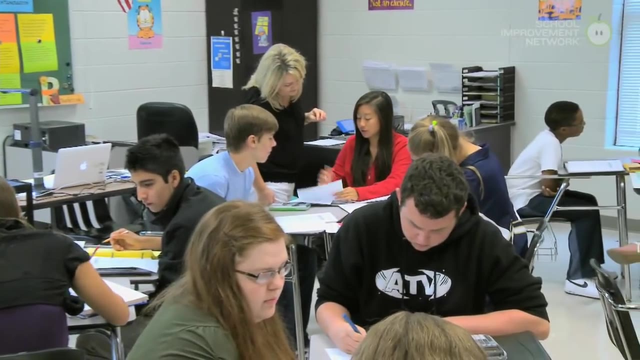 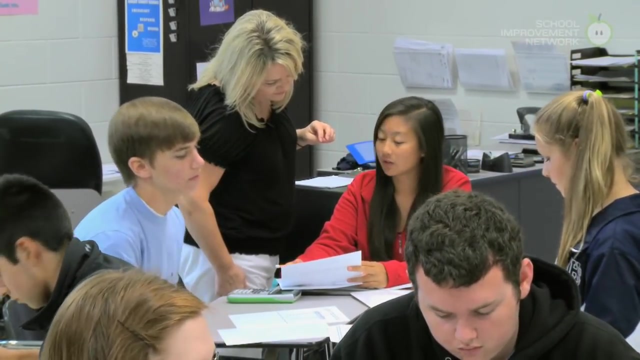 Y'all think about this graph. they're all doing Yeah, Like that Mm-hmm For the years, like do we go from tens? can we do that? Or do you want us to literally write 9.8?? 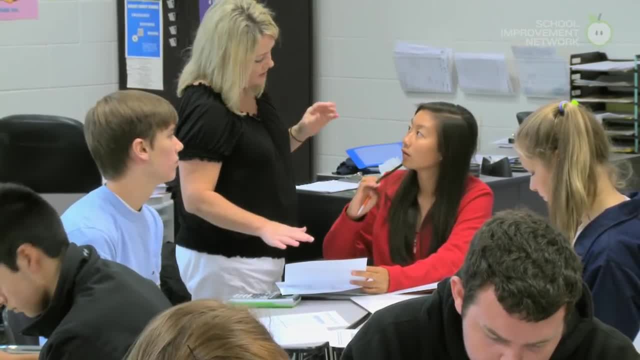 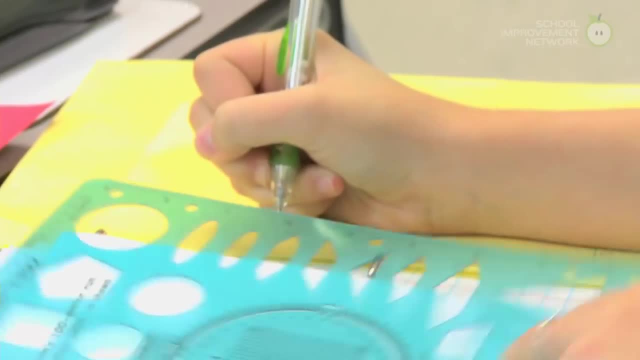 Nope, You can do whatever you want, Okay, Just remember, you're going to type it in the calculator eventually, But no, you can count by anything you want. Okay, And it goes up to 11.. Mm-hmm, So is that okay? 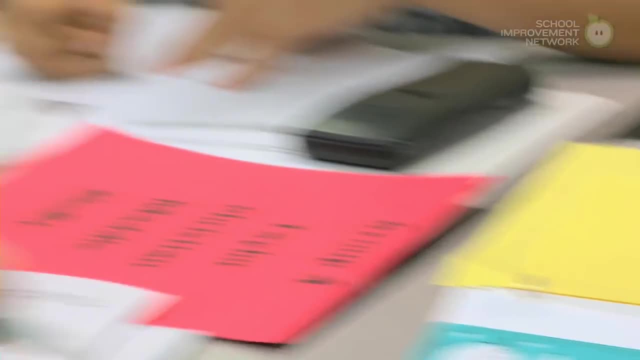 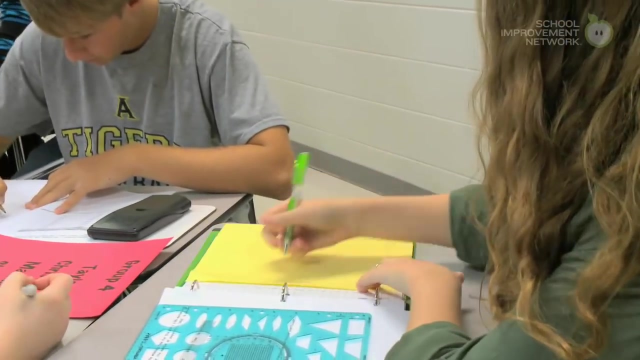 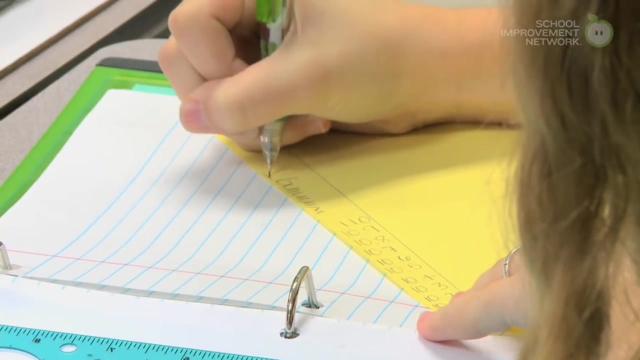 Yeah, I would actually see how it puts .0.. So when it says 10 and 11, I mean it's the same thing, but just to make it even. And then it says: Did y'all decide on a scale? 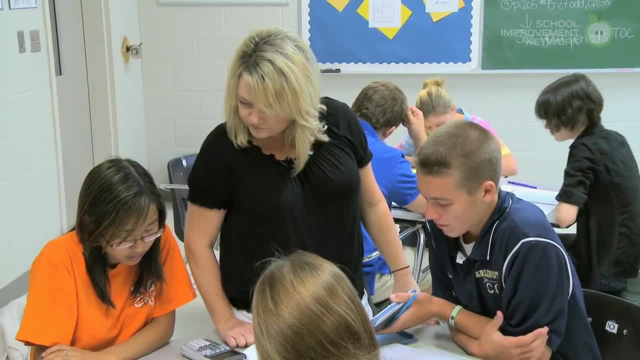 Yeah, we're going to go by 12s on this one. We can't really figure out like what. Okay, We're going to go about like 116 units to do that, so Okay. 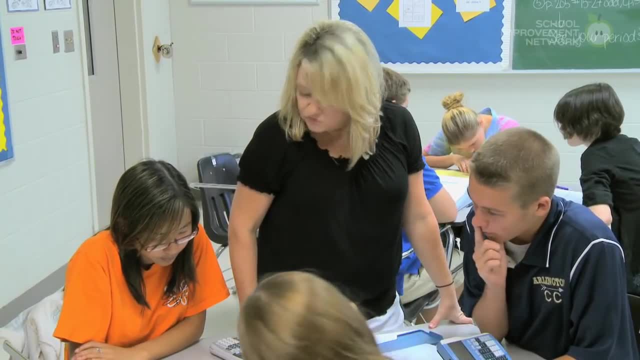 So where do you want to start? maybe 9.8.. 9.84.. You're starting the exact, Yeah, Or maybe a little bit further than 9.8.. Can you do a squiggly line for the x-axis? 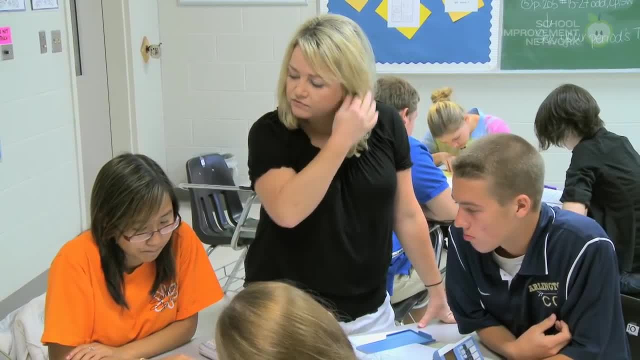 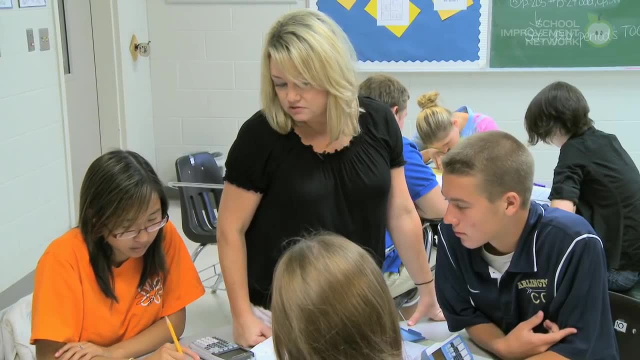 You can Do you need to, though. Do you need to do a squiggle? What's that called Squiggle? A break, Mm-hmm. Do you need a squiggle on the x or do you need a squiggle on the y? 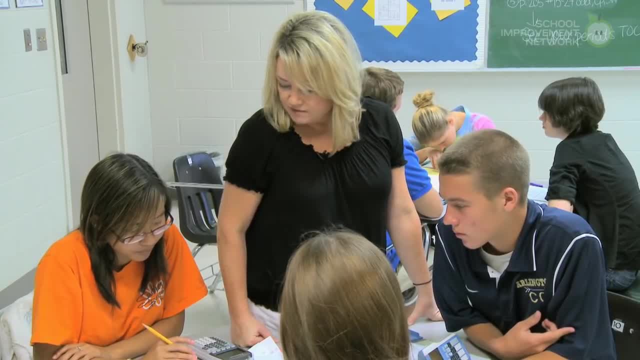 Y, Maybe the y, not the x. Mm-hmm Y, What are you going to start with? on the x 9.80 or something? No, on the x-axis, The x-axis, The 1900.. 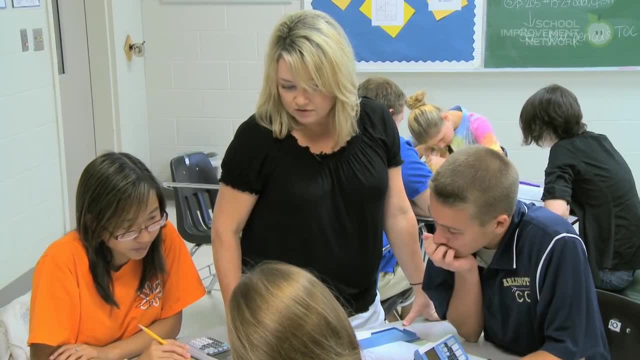 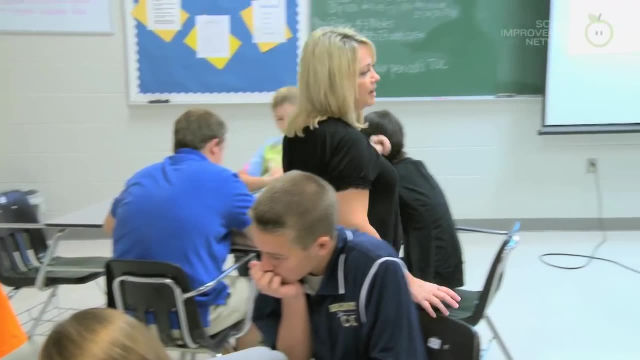 So there's really no break there, Okay, but you do have a break on the y-axis. Good, Good, good, good, And you've got a good label. I'm going to pass around some questions that you can use to help make sure you're on the right track. 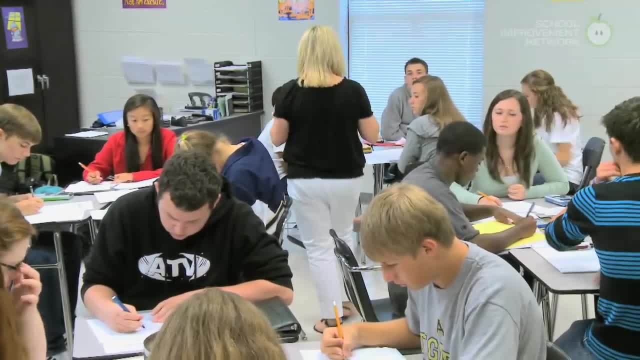 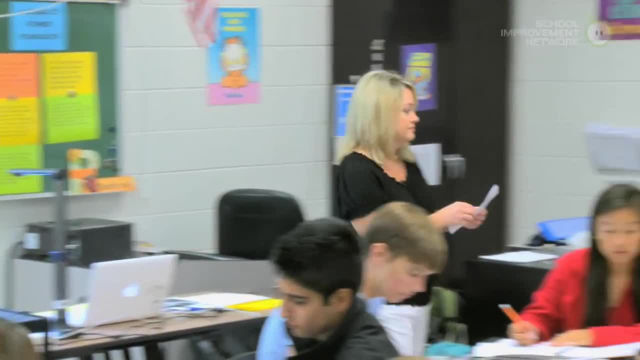 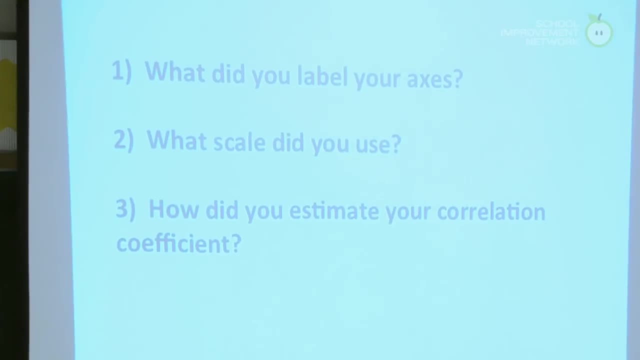 Okay, Just a few little questions to think about as you're doing this. Yeah, absolutely, You can write on these questions if you want to, Just making sure you're doing that. We're going to do that in a minute, okay. 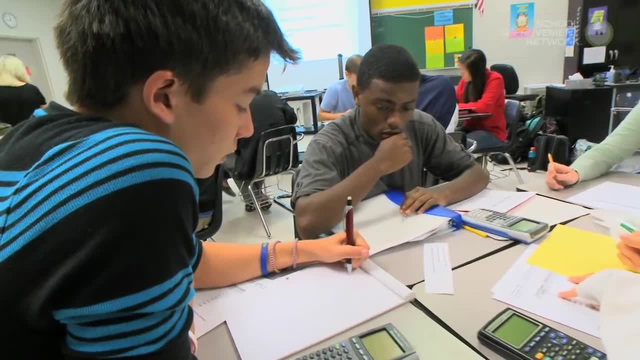 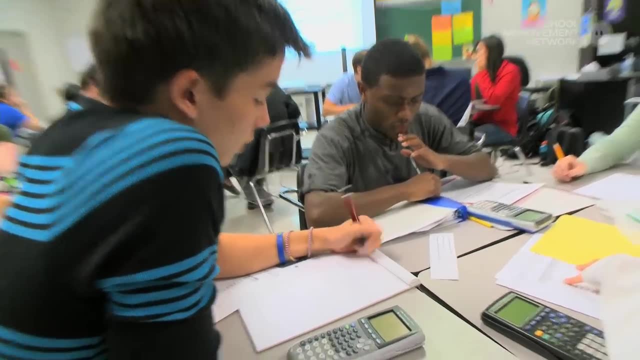 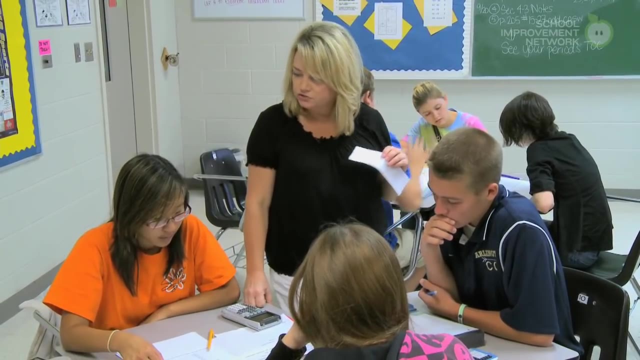 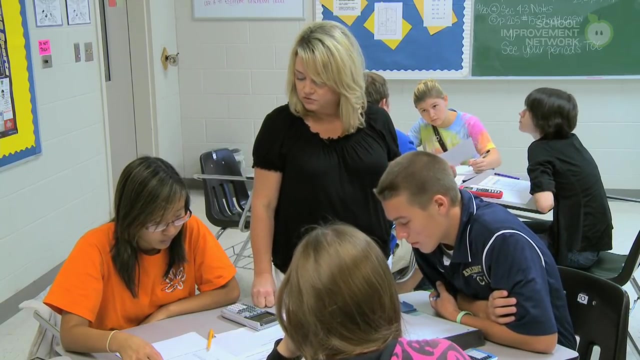 Yeah, Okay, tell me a starting point. Where could you start? Do you have to start at 9.84?? I'll start at 9.84.. Okay, you can start at 9.8.. And you've got to go to what? 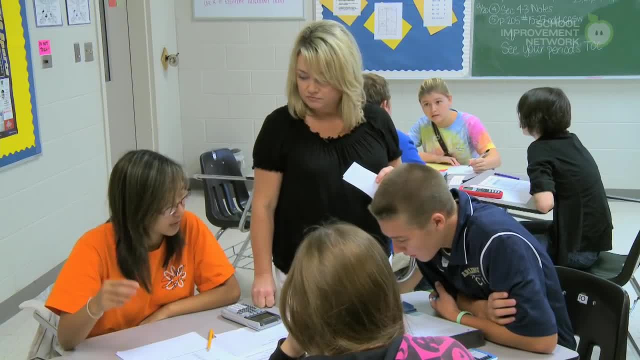 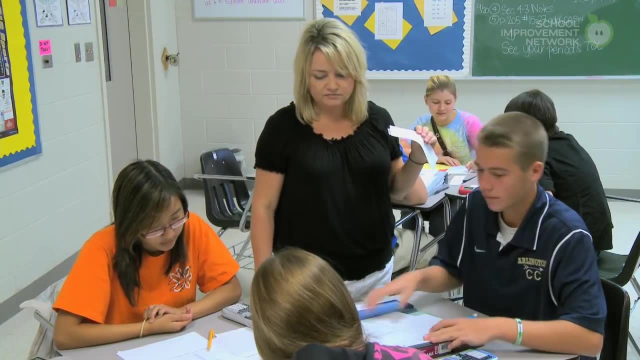 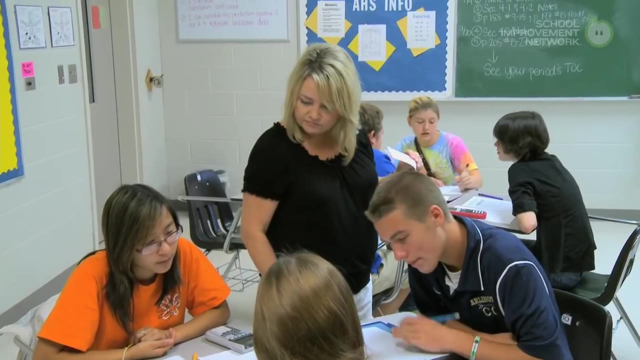 11.2.. 11.2? Or 11?? Let's go by .2.. Okay, perfect, As long as you're consistent, as long as you label, there's not really a right or a wrong. Yeah, 9.8.. 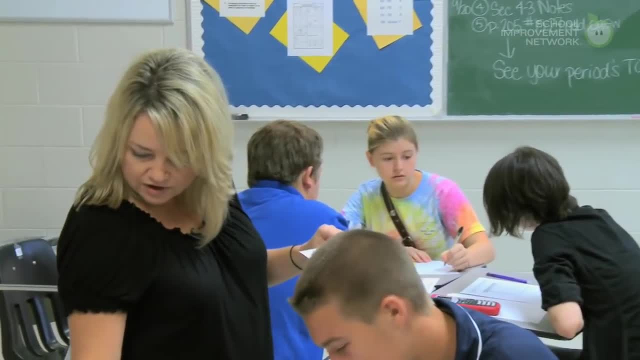 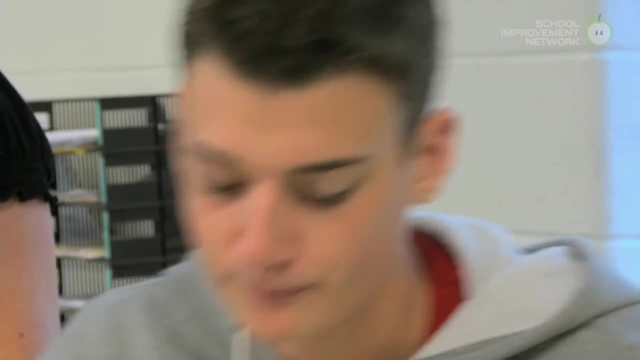 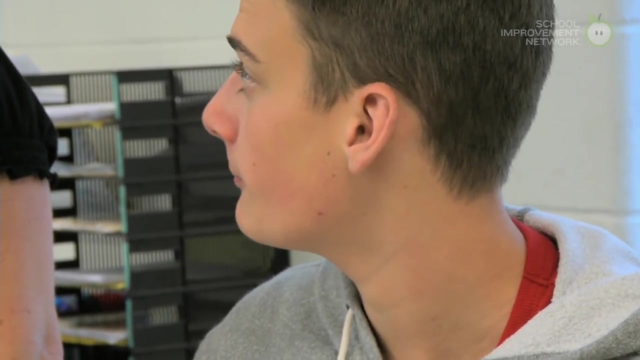 And then think about these: okay, Okay, Wherever it goes, it goes. It doesn't have to do a specific thing. okay, How do you know it's going to make a line and not a quadratic? Wait, what do you mean? 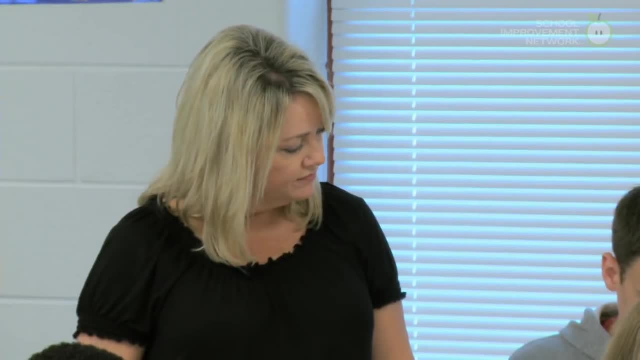 Like, how do you know that's going to be a line that you're drawn through it? Can you tell that? Because it's all it's, they're not all spread out, They're not all spread out and there's no curve. 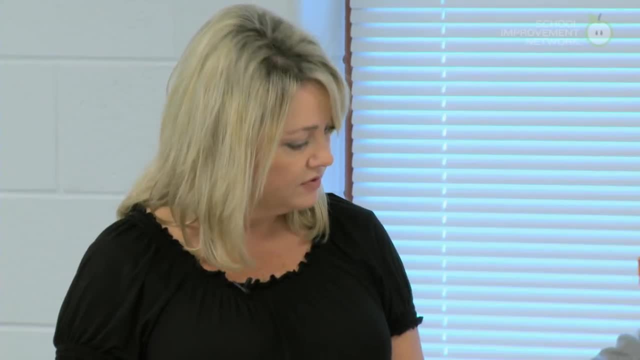 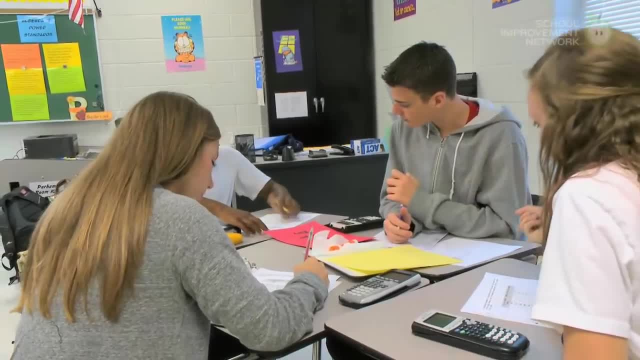 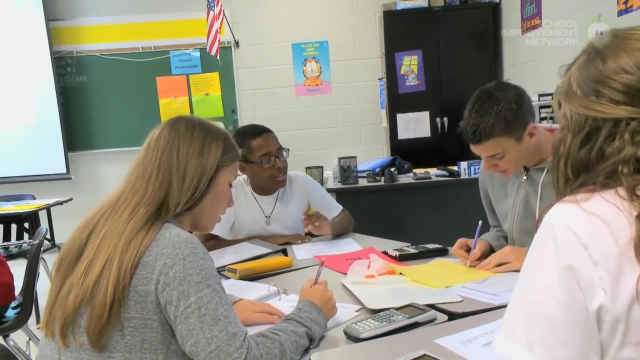 All right, Okay. So Wait what The winning time? T Okay. And then, years Between T and Y, We thought we were just going by the axis. Yeah, so we could just put like. Put it like in parentheses. 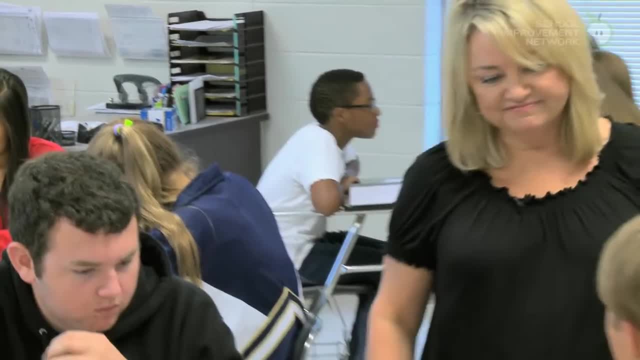 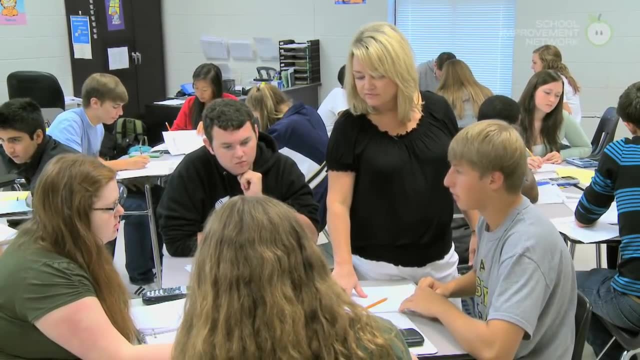 Well, Do we all have to do these questions or do we just put them separately? No, you can all answer together based on your yellow. All right, So just have you all done all of these. We are going clear now, right? 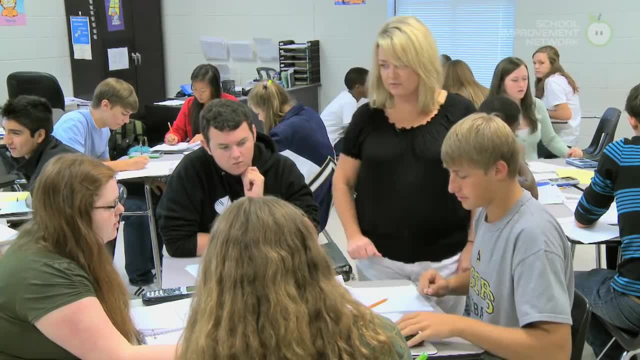 Mm-hmm. And when you decide on your correlation coefficient, I want it on the whiteboard, But don't let anybody see it. All right, is that going to be on a notebook paper or are you going to write it on the whiteboard? 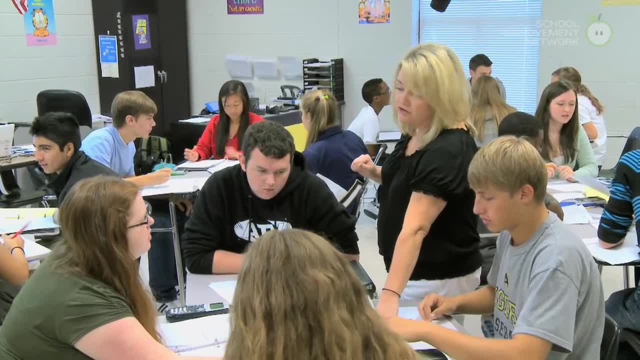 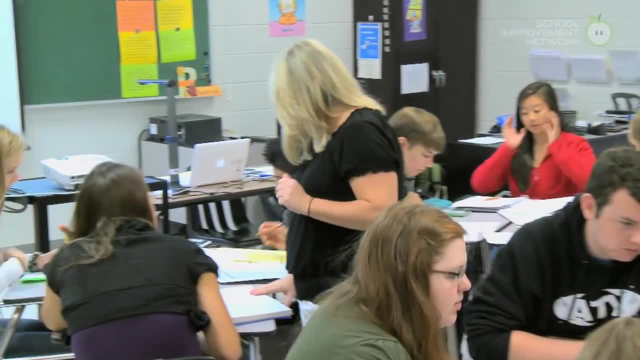 No, you can just do it right there. This is just making sure you've done everything. You don't actually have to write it. Oh, all right. Okay, It's just help make sure you've completed everything. Nice, Nice. 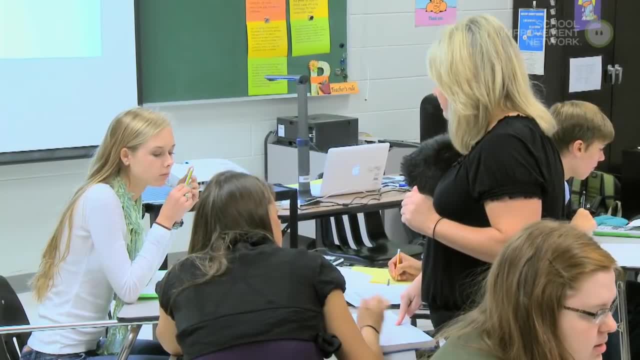 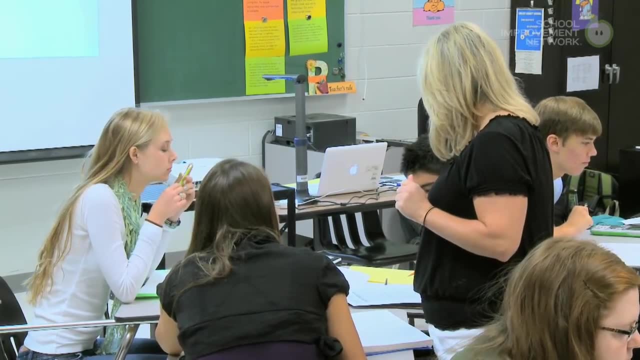 Okay, tell me how you knew this was a straight line. There's no, what Huh? There's no curve to it. Mm-hmm, Perfect, No curve. So you knew it was linear, right? All right, Have you all estimated your correlation coefficient? 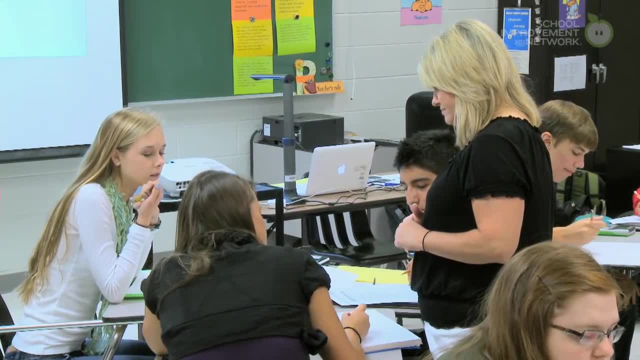 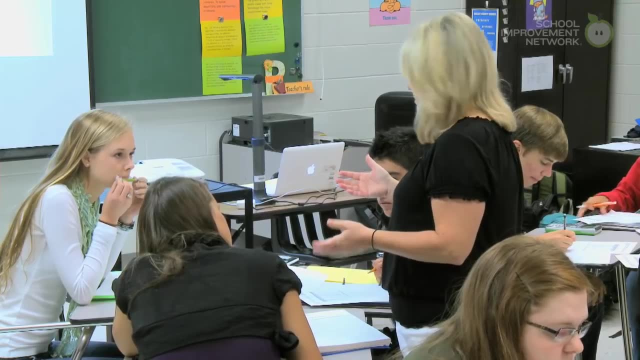 We did Like would this be? Is this part of it, though? Would we even look at this part? That helps you decide. Remember what's a perfect correlation coefficient: One or Negative one. Negative one, So the more points away from it, or the farther away, the closer to zero. 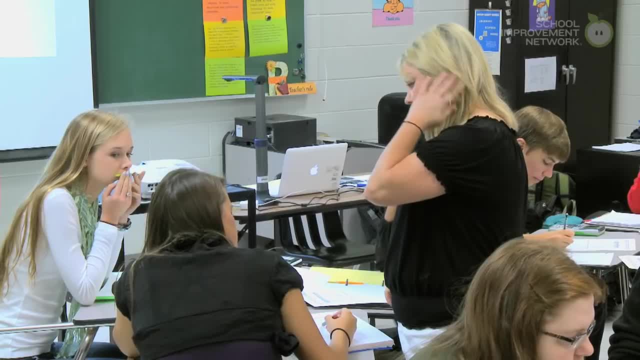 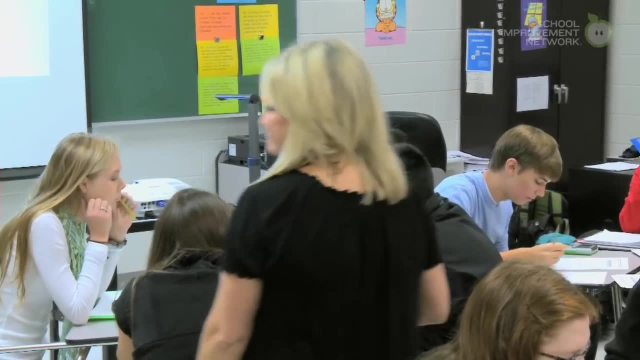 So you're going to kind of guesstimate, Wait. so these would also, these would have an effect on the line though. Yes, Okay, Yes, Mm-hmm, Mm-hmm. Hey guys, How are y'all doing? 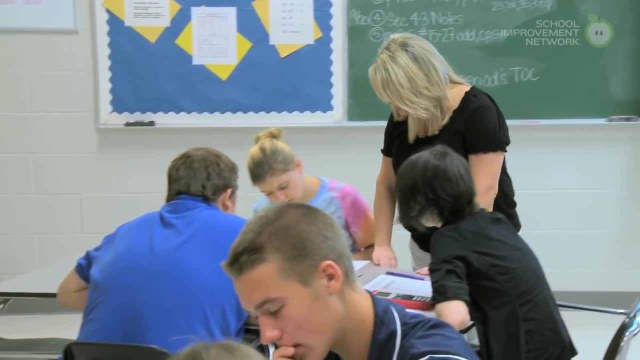 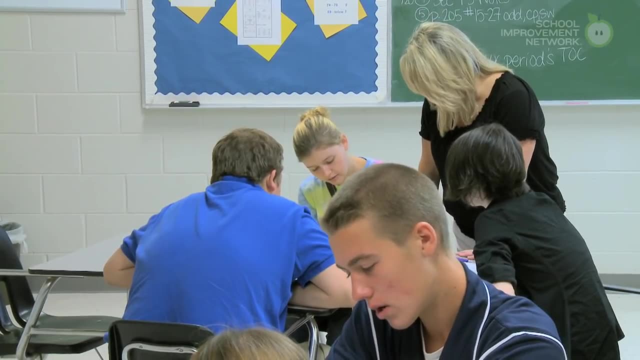 Good, Good, Good. Did y'all go through your questions? Yes, ma'am, Yes, ma'am, Yeah, Okay, Are we ever changing our prediction now Because she made a mistake? Yeah, I made a mistake. I put it under 1020 instead of under. 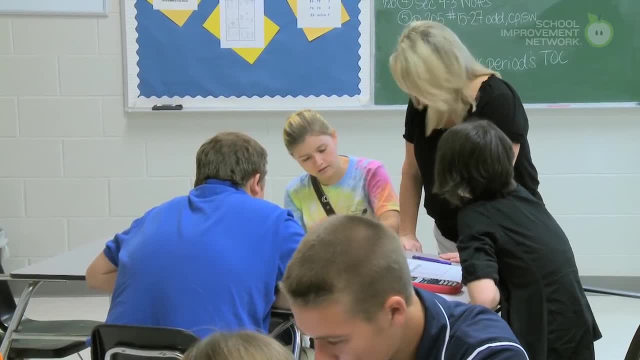 Okay, I mean, it's not 1020.. So it might be a change. It's still a strong net in correlation. Yeah, Okay, I'm thinking. no, I'm agreeing with you. I'm thinking, no, It's like negative .9.. 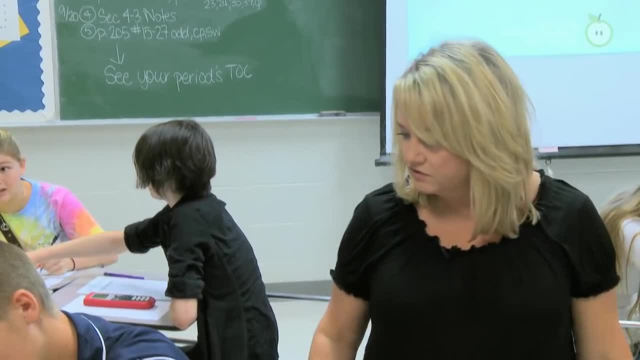 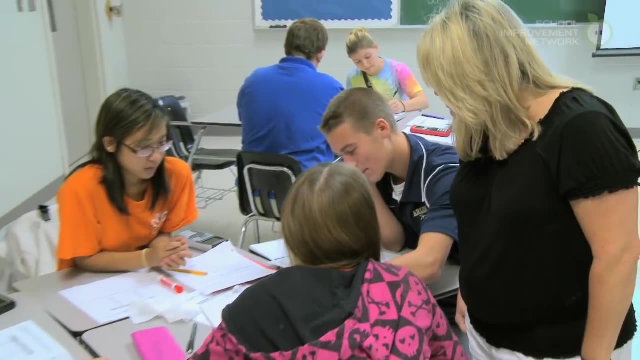 All right, When you're set, put it on your whiteboard. Okay, I think y'all are good. I think we got this one Closer, Closer. All right, You're a perfectionist at this table, aren't you? 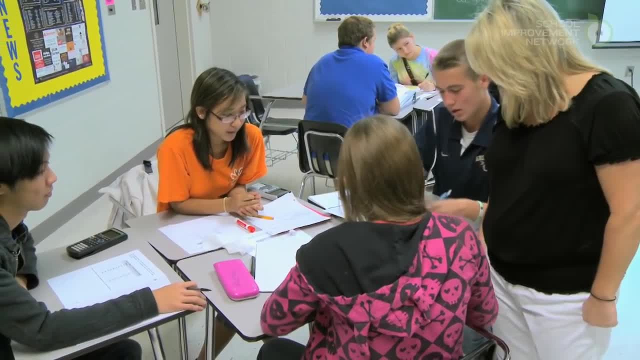 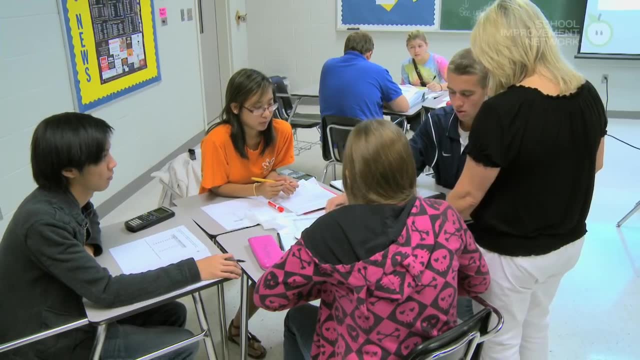 Yeah, Yes, I like it, Nice, Okay. Okay, Let's talk about what type of function this is Negative. Does it have any kind of curve to it? I can't see it. It's a Kind of. 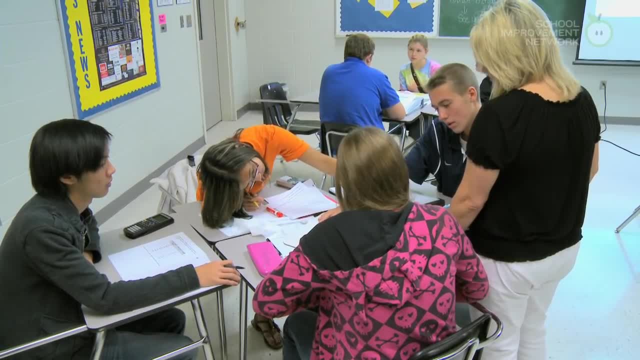 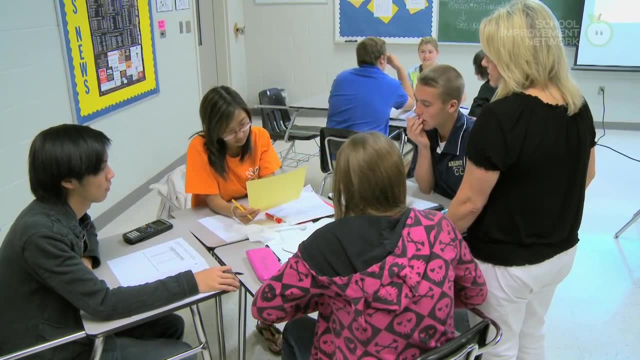 Because you've got to decide what kind of function Linear You think it makes a line. Yes, ma'am, I would probably agree with you. It doesn't really curve enough to make any Make it anything different. No, 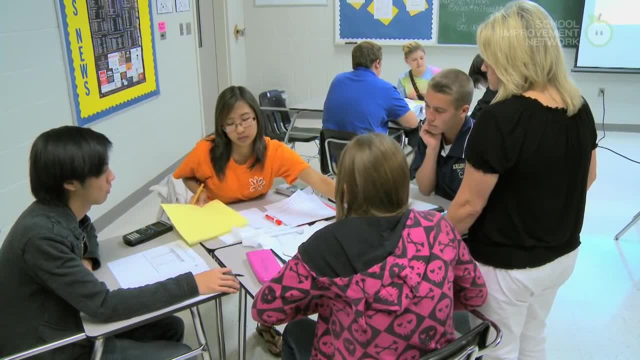 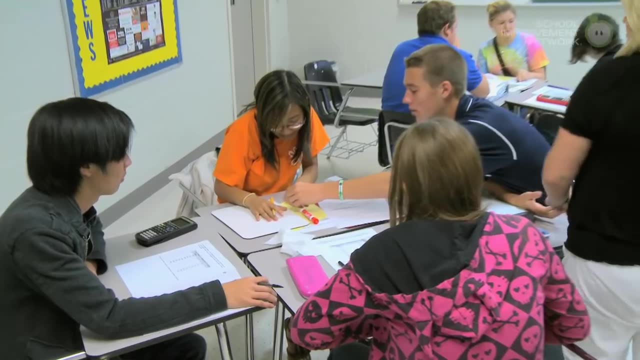 Yes, ma'am, Mm-hmm, Yeah, Because. So draw the line you think has the best fit to that. Draw This line, This line, And Nice, Nice, Nice, Correlation. 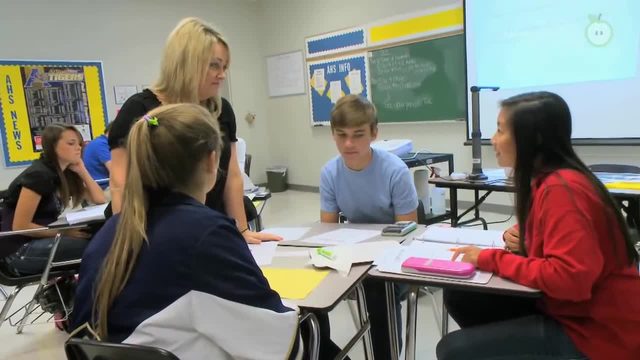 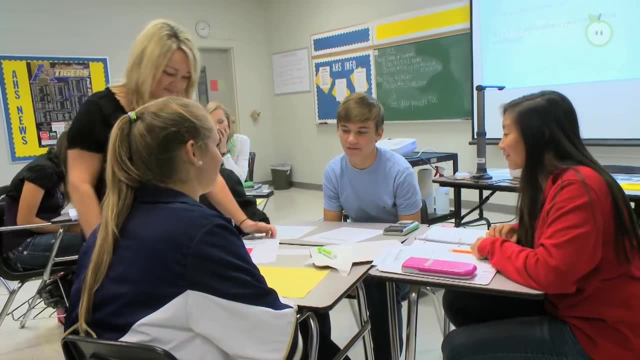 A whole line. And what is that one? What's that called? That one lonely point out there, What is it called? It's like Good, Good, Good, Good, Katie, Good Maria, All right. 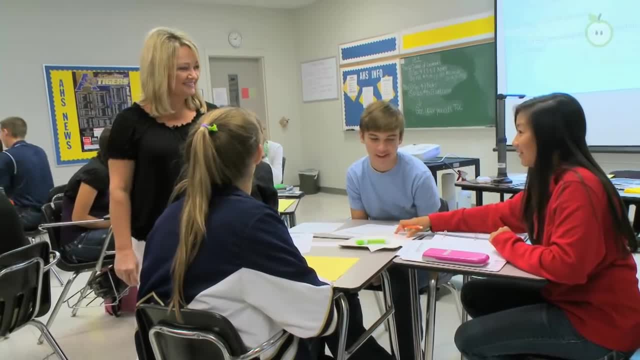 You're all going to come up with your correlation coefficients. You want the press, don't you? We really do, Yeah, Thank you. Did y'all go through all your questions? Mm-hmm? Yes, ma'am, Yeah. 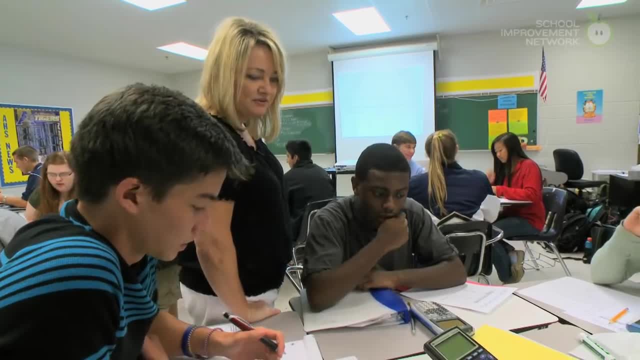 Have you come up with your correlation coefficient yet? Yeah, we have. Okay, Will you put it on your whiteboard for me? Okay, And we're going to hold them up in just a second, Just. That made me really off. 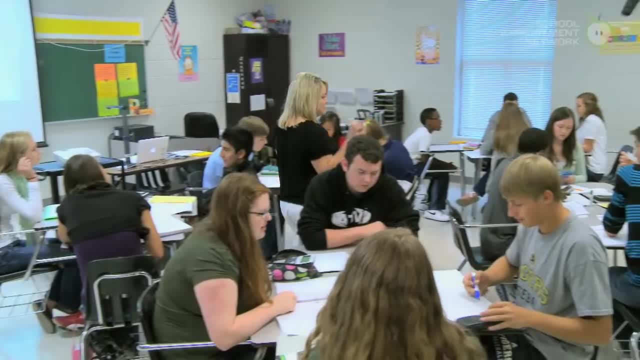 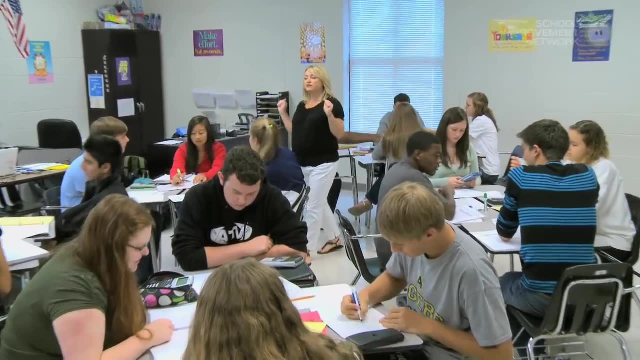 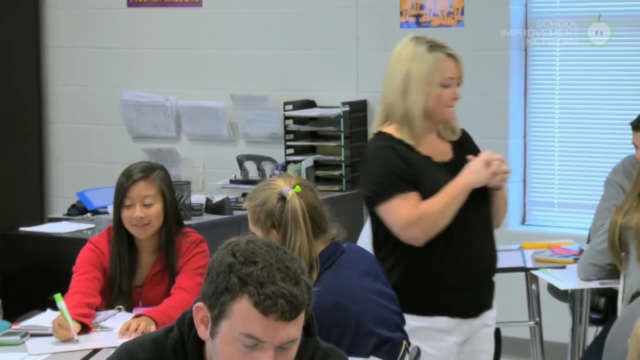 Okay, Okay, You have about 10 seconds, Ten seconds, And I'm going to ask for them. Wait to the thousands. Yes, Yep, I want it to the thousands. 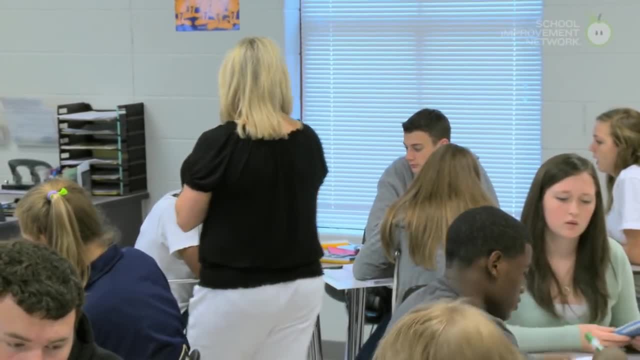 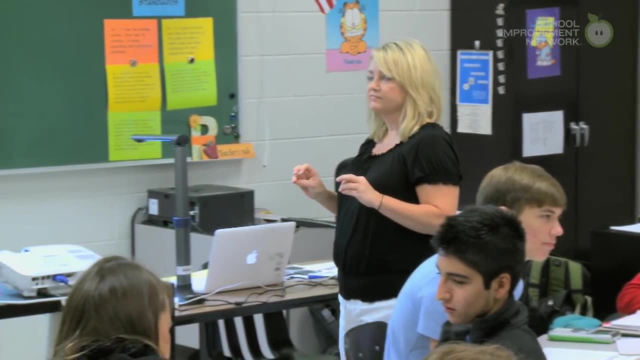 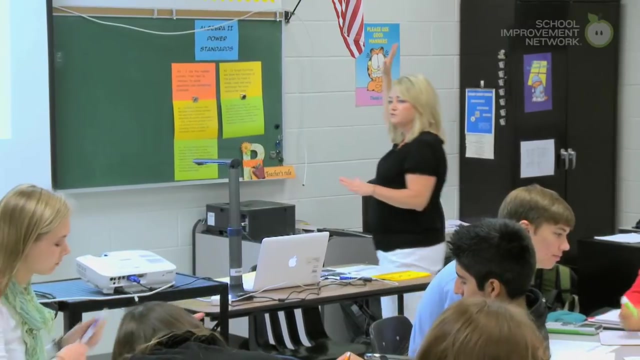 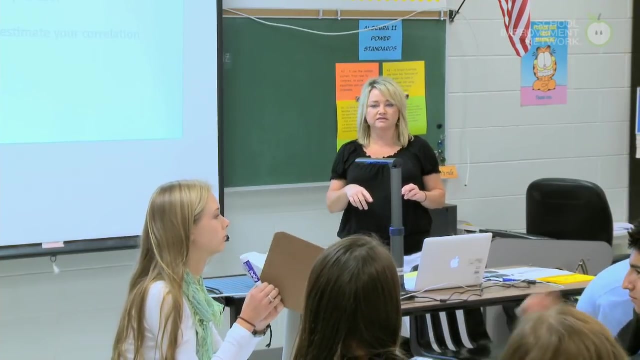 Okay, Can I have everybody's attention up here? Let me see those whiteboards. Let's see what we've got: Negative .987, negative .974, negative .85, .957, .965.. These are. 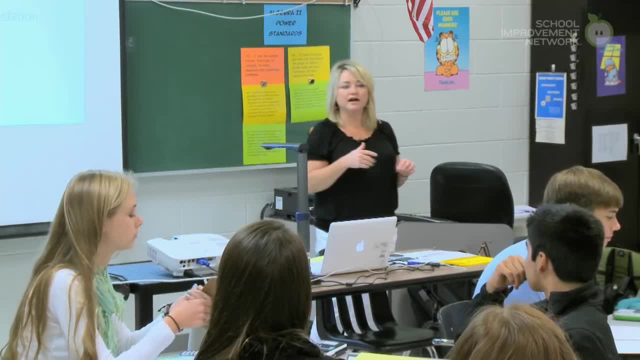 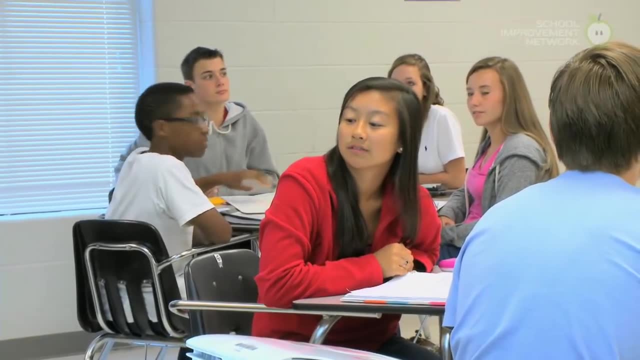 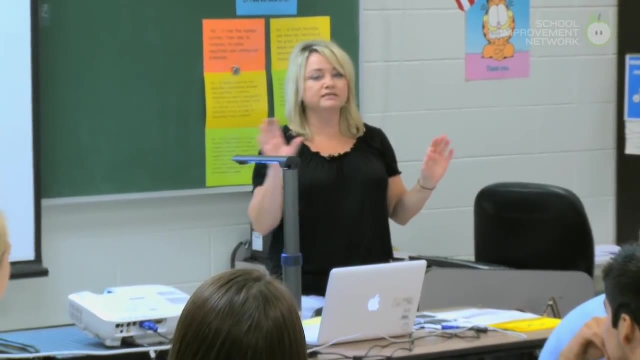 very, very good predictions. Who can tell me why everybody has a negative? Raise your hand. The line is going down. The line's going down. So if your slope's negative, your correlation coefficient's going to be negative as well. Okay, so somebody tell me who wants to show. 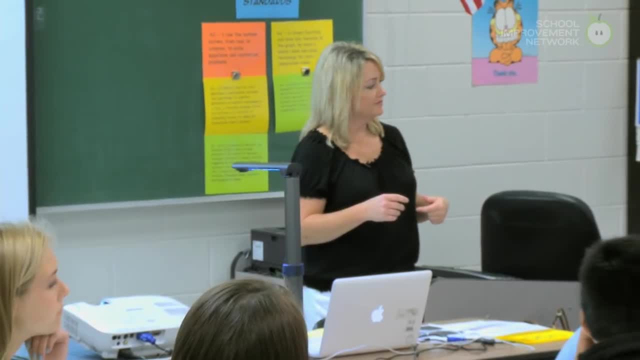 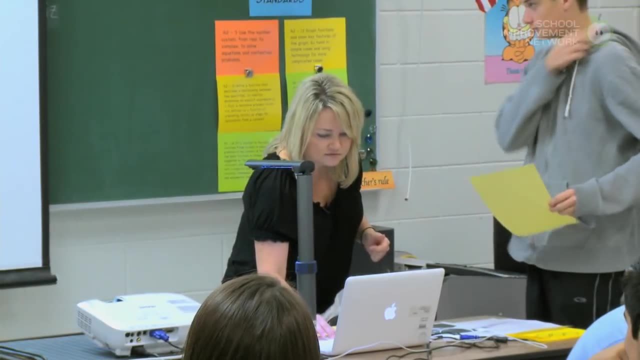 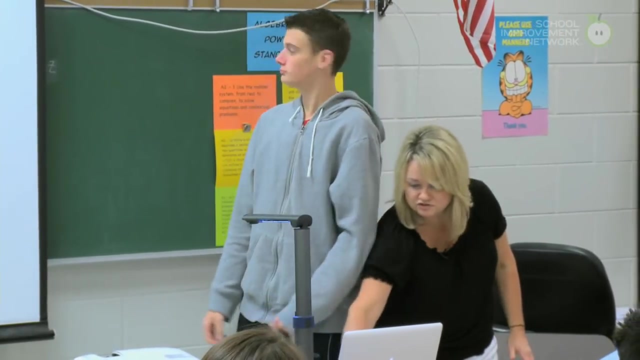 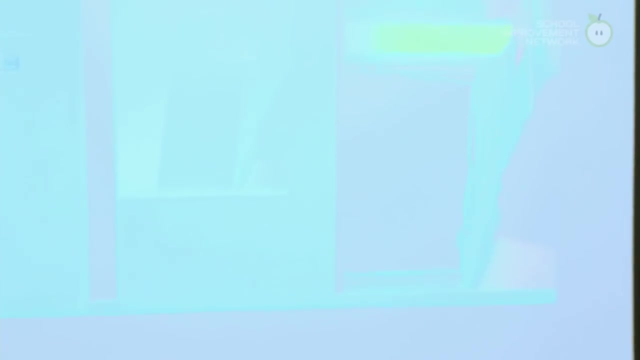 their graph. Riley, will you bring it up here for me? Just let me move this for just a second. Okay, Set it right there for me. Let's see it. If it's going to show, We'll get there, We'll get there. Okay, So here's their group. That's pretty good. So you let your x-axis 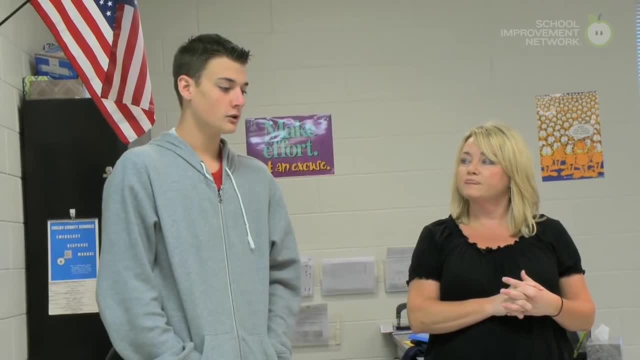 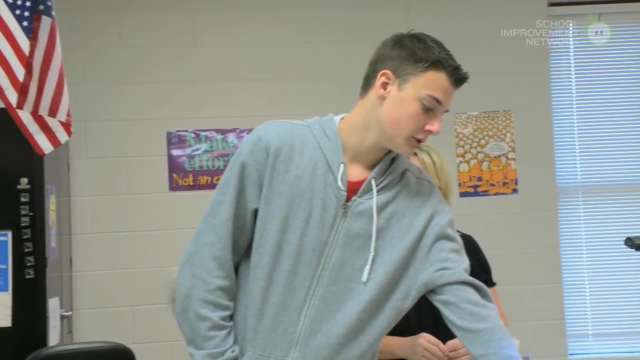 be years. Yes, ma'am. Okay, Why'd y'all choose that? Because it was an independent variable and like how I had to explain it to my group: the time is dependent on the years, not the years dependent on the time. 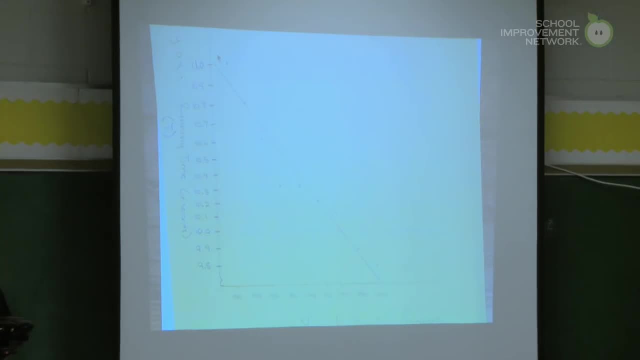 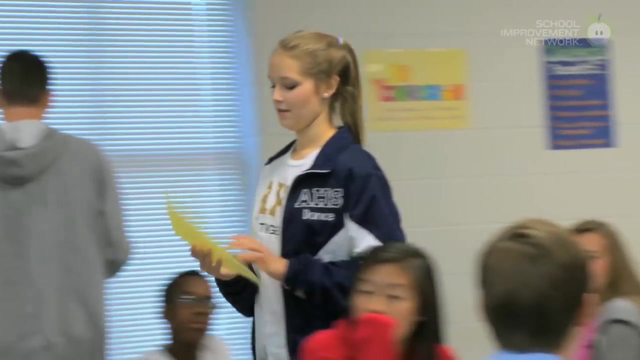 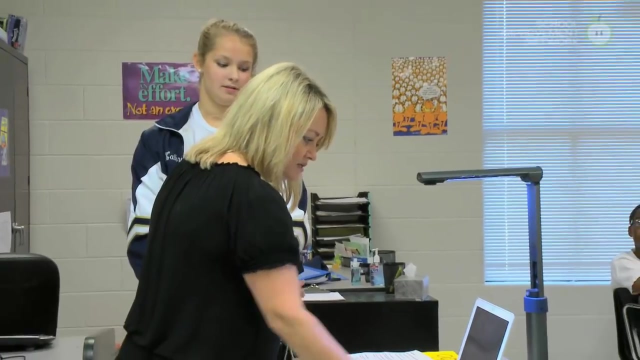 Nice, Very nice, Very good graph. I like it. Katie, you want to show yours? Thank you, Riley, Take that map. Oh, I see You did years, But they didn't do the exact year. They did their years by tens. 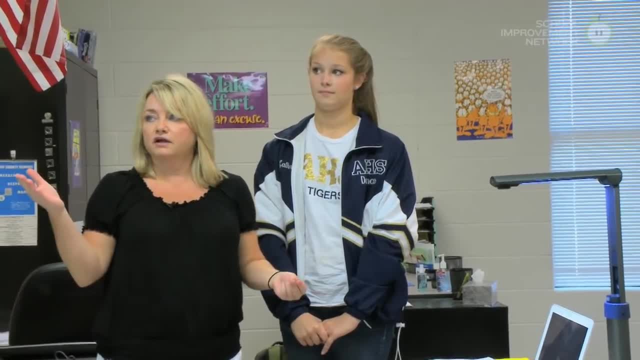 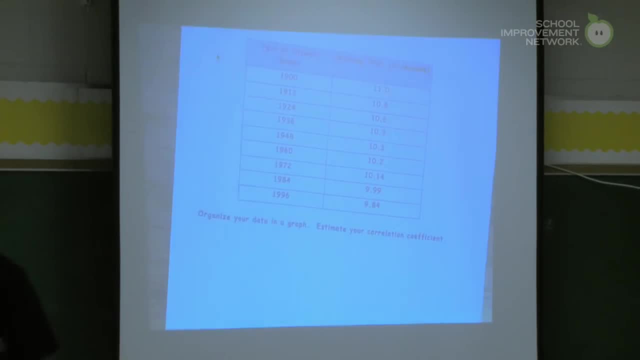 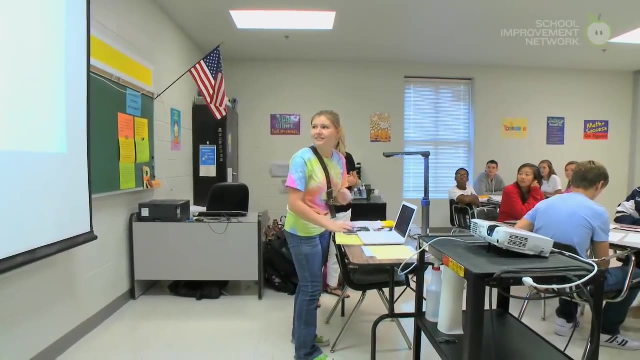 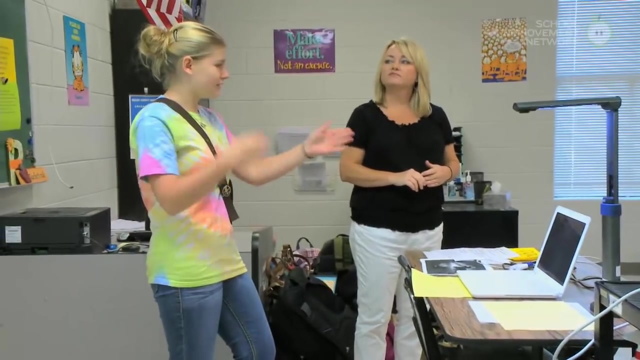 Is that okay? Yeah, Nothing wrong with it, right, As long as it's labeled. you're good, Anybody have something different Parker. Thank you, Katie, Nice. Why did you choose to use two digits for your years? It was just easier than writing out 1,900,. 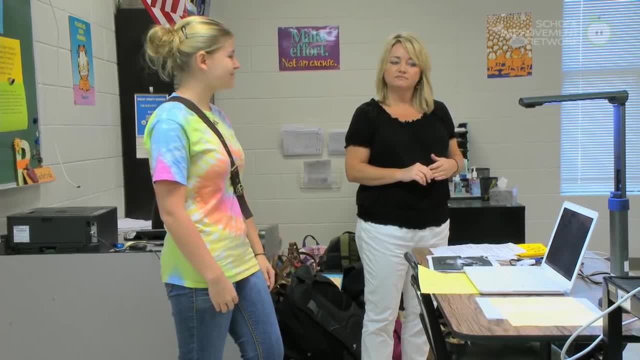 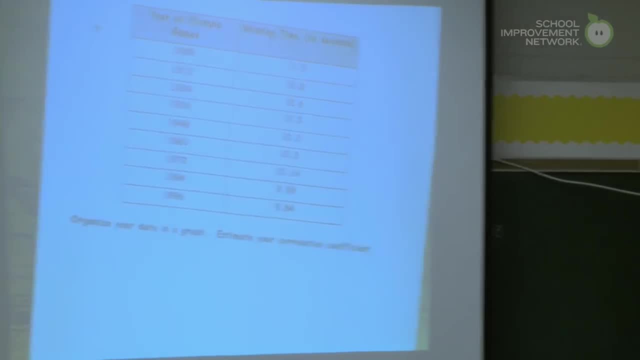 and it just kind of simplified it for you. Okay, Awesome, Thank you. Okay, How can we check our graphs using technology? What can we do? Amanda, You could use your calculator and do stats. Awesome, Okay, Let's do it. Let's use. 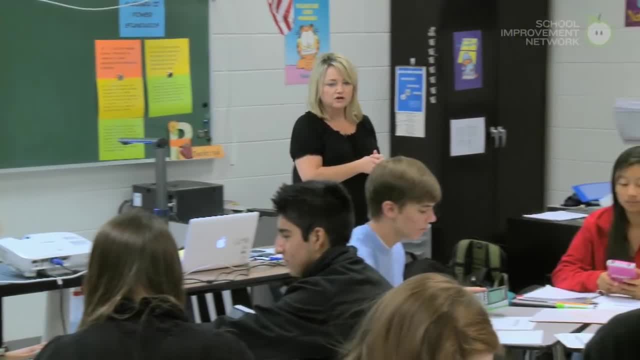 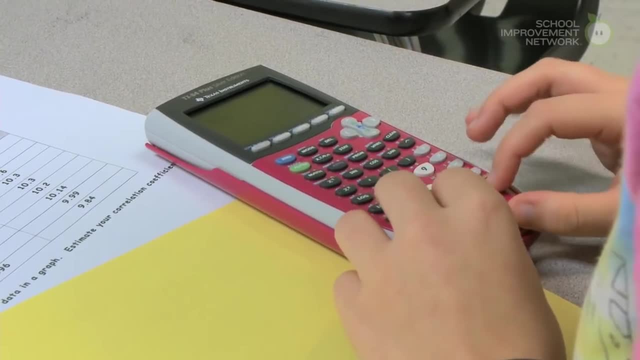 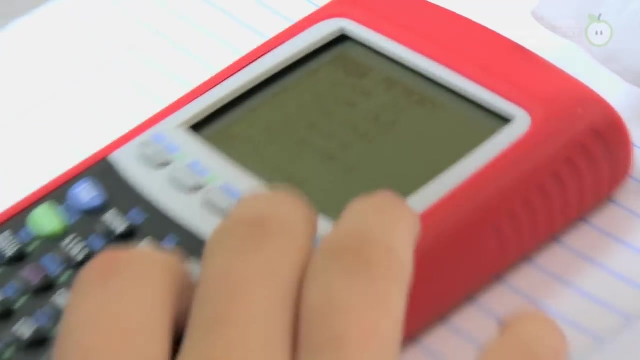 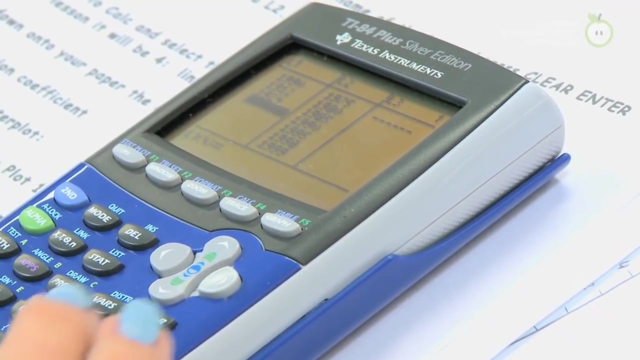 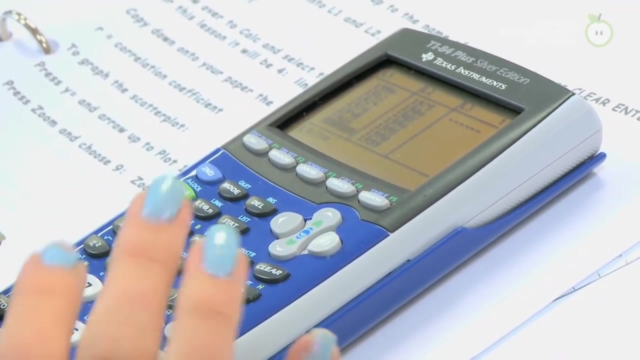 your calculators, enter your data and let's draw our stat plots. Kathie, Yes, Great, That's it. Okay, that's it, It was easy. Okay, let's go ahead and try this again. I wish I could do this next, but I can't fully see anything. 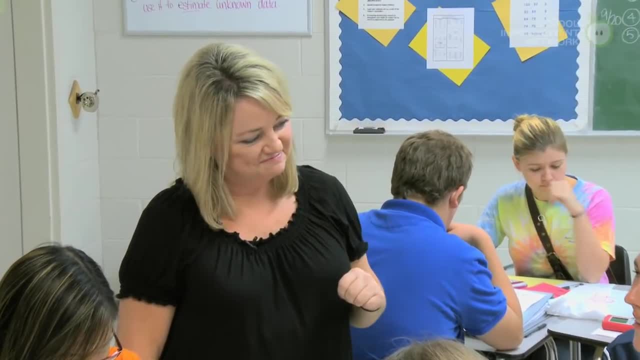 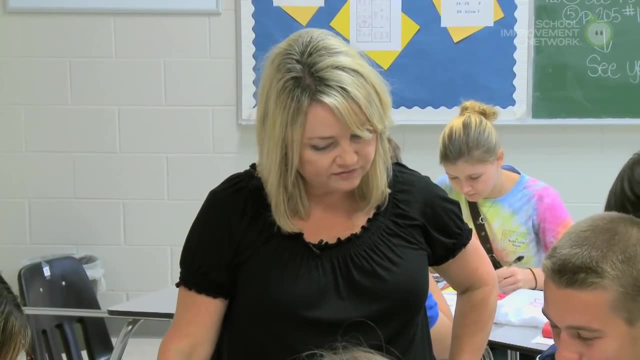 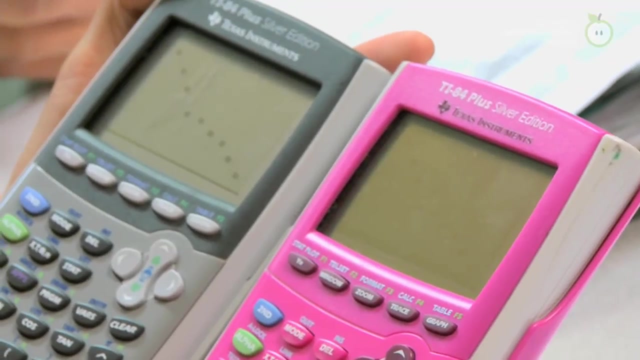 mu medieval. Why? Okay, Not yet, That's your regression. Zoom stat, Zoom stat, Because all your data is in your stat. Good Good, good good. I see some of you started at zero. 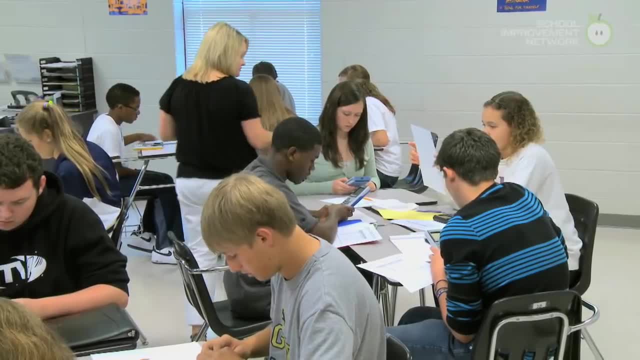 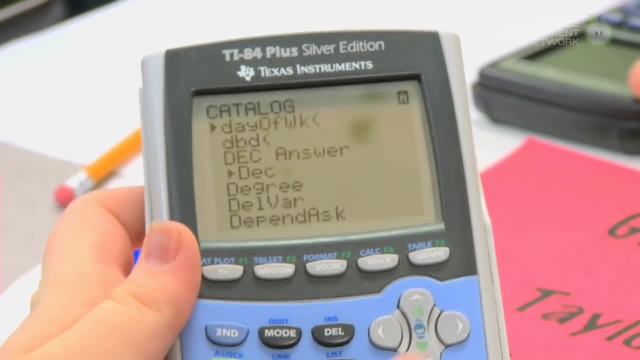 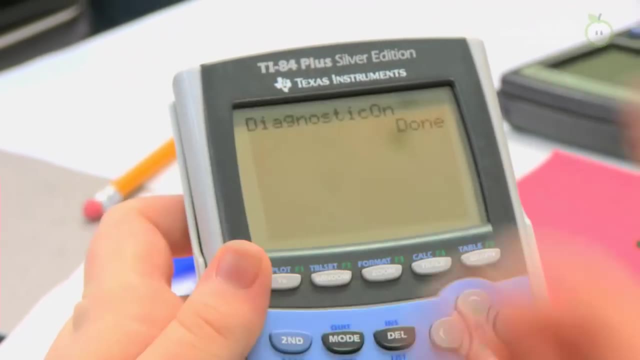 Some of you are using the full year. It's good options, Good options, Mm-hmm. Okay, Yeah, we want to graph first. Okay, Hey, y'all look up here for two seconds. We've got some questions on graphing. 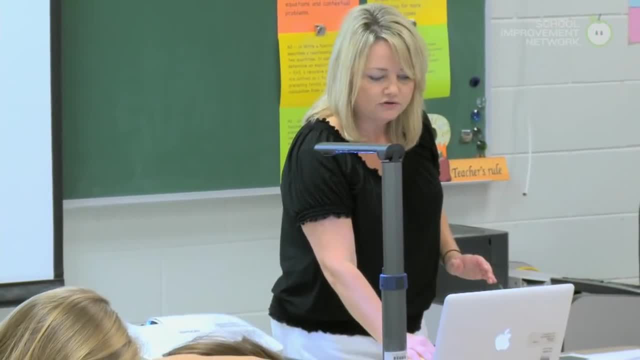 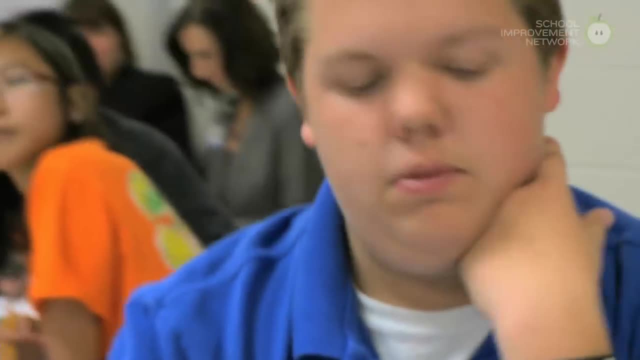 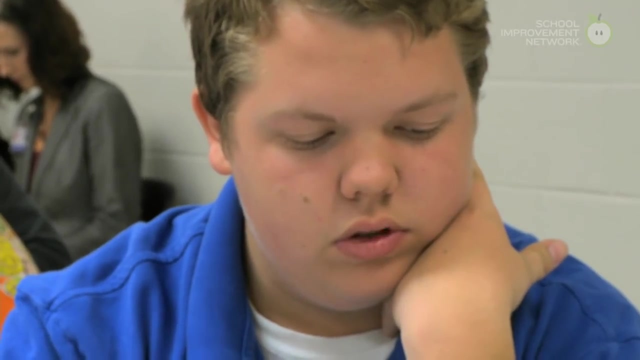 Once you enter your data into your calculator, where do I go to actually see it on my graph? If I want to see the picture Will Push zoom and then push nine, Zoom and nine. And what is number nine? That would be zoom stat. 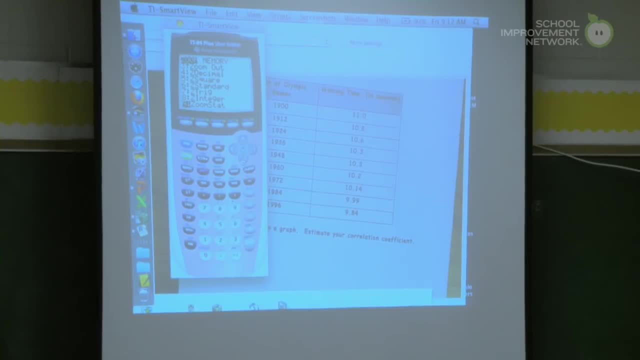 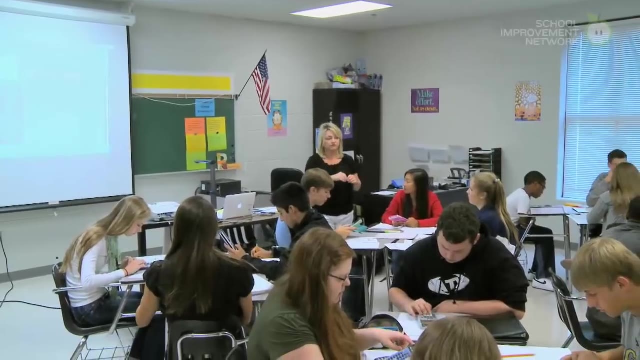 Zoom stat Because we went to stat to enter our data. So zoom stat is going to show our graph. Why could it look a little different on the calculator than on your graph? The scale's different. The calculator's a lot smaller than your piece of yellow paper. 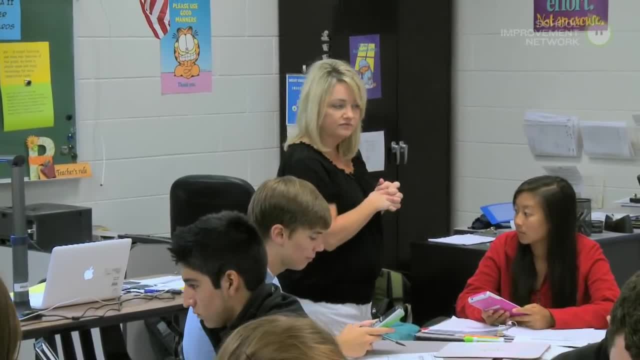 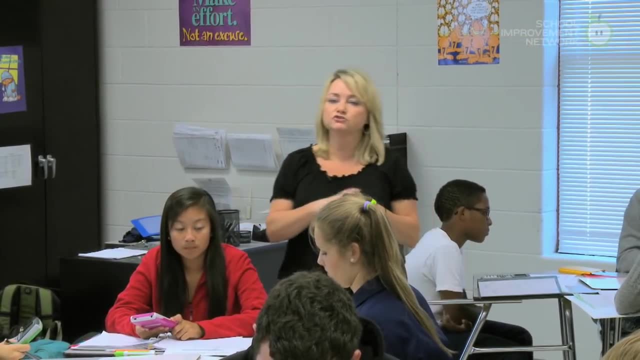 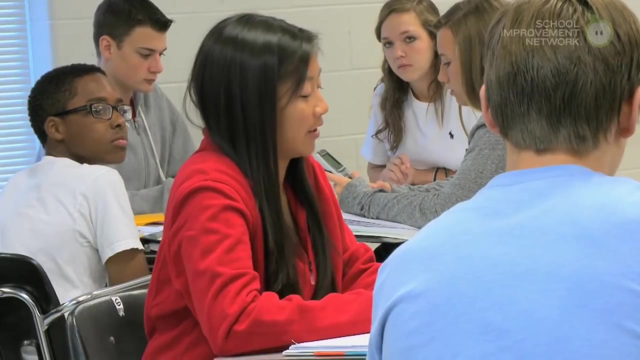 So, depending on the size that you drew? Okay, So how are we going to test our correlation coefficient? Where can we go to determine what it really is? You click stat and you arrow over to calc and then go to the line. We know this is a linear function. 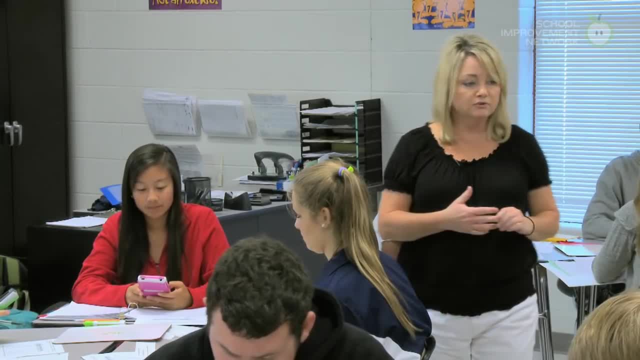 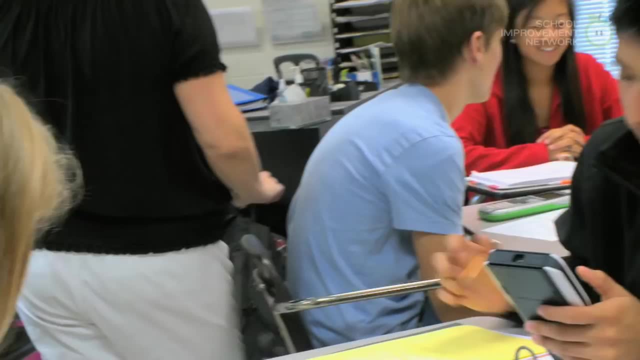 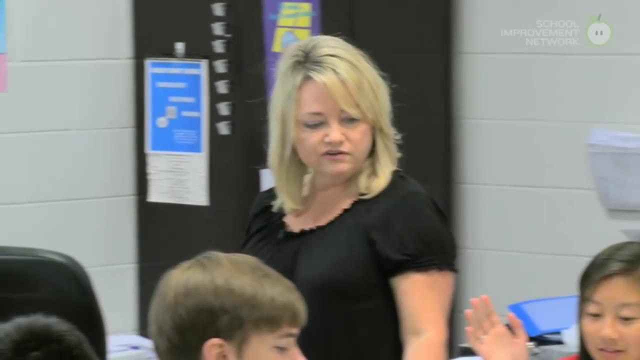 So we're going to do our linear regression. Okay, So do your linear regression and let's see who got the closest to their correlation coefficient. Who thinks they got the closest? Who got the closest? Y'all think y'all are close. Let's see what it really is. 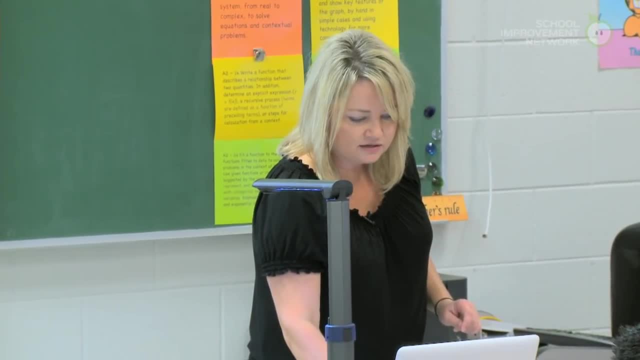 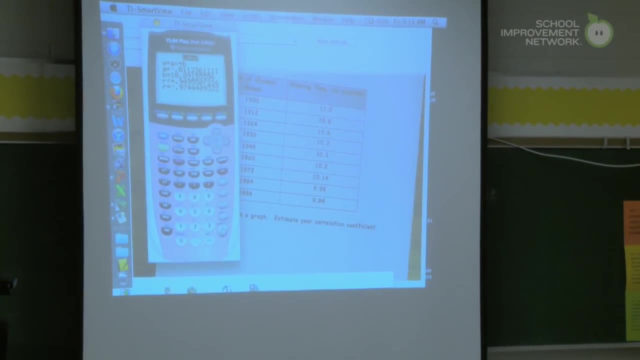 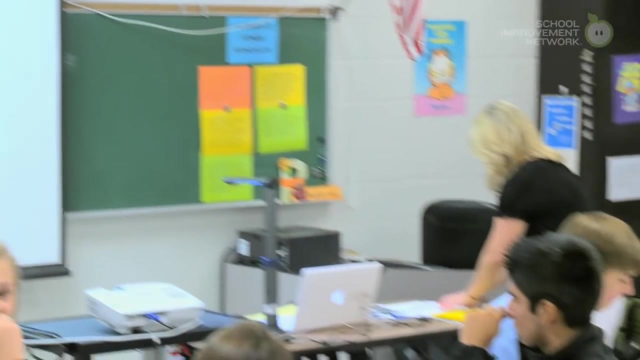 Did you get it? We did a stat. We did a stat. We did a stat. calculate linear regression: Negative: .974.. Who thinks they're the closest? You got the exact one. Awesome, Guess what you win? How about a gold medal? 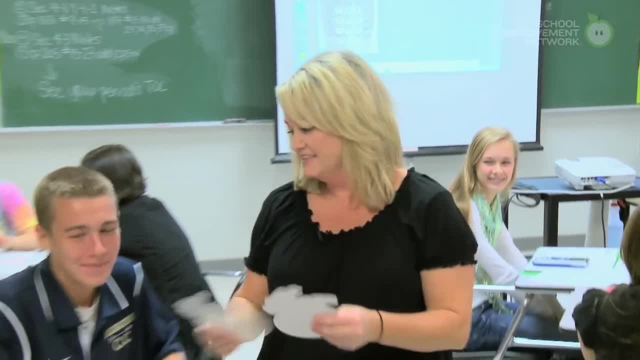 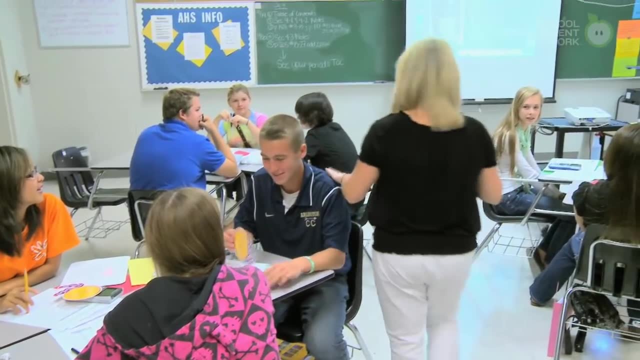 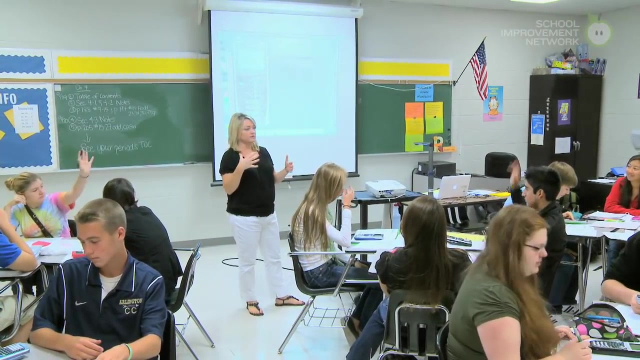 You've already won your gold. Awesome. I apologize, but I can't sing the National Anthem And you probably don't want me to sing the National Anthem. Okay. Who can tell me what else we can use this linear regression for Ricardo? 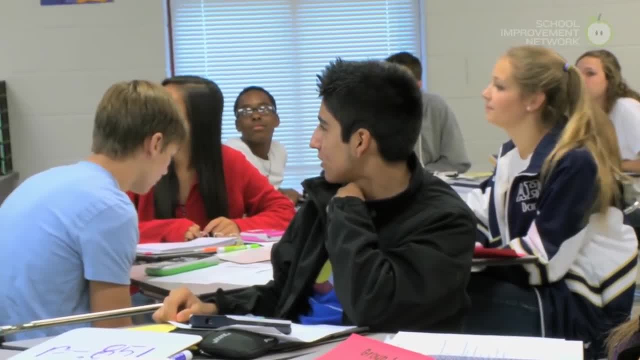 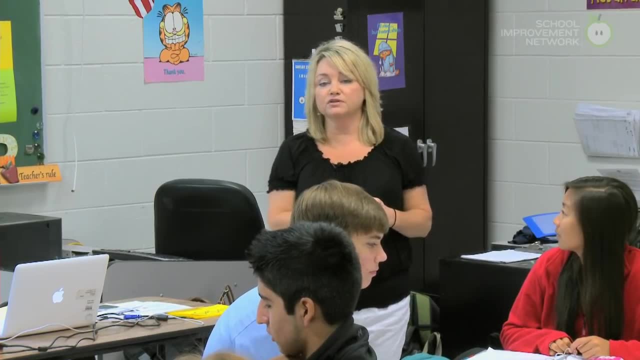 To make predictions. Okay, To make predictions. What data do we have now that we didn't have before? From your calculator, A prediction? I'm not sure. Coefficient Parker, The prediction equation- Perfect, So I can use the prediction equation. 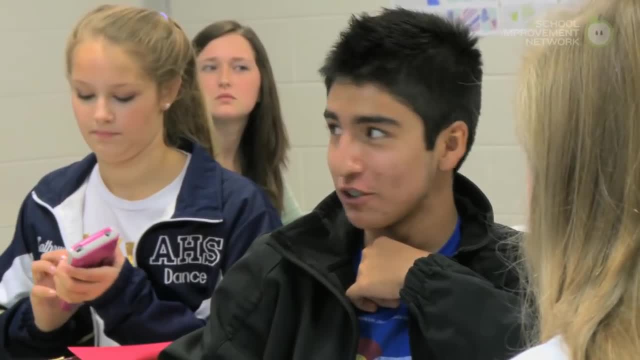 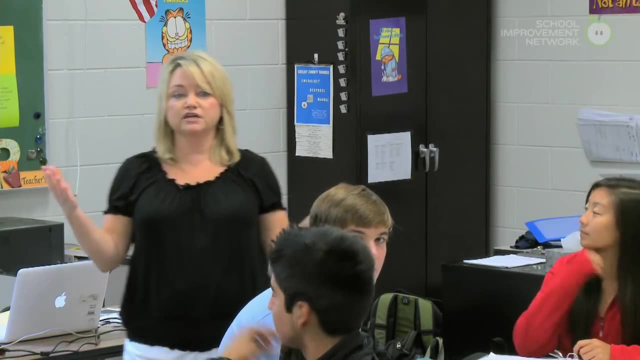 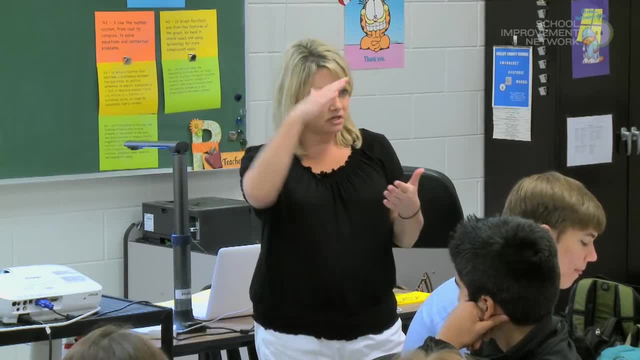 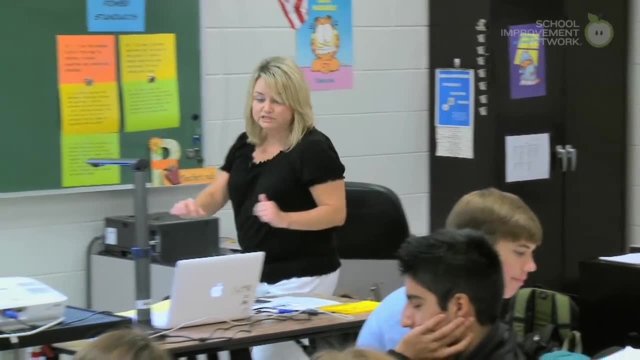 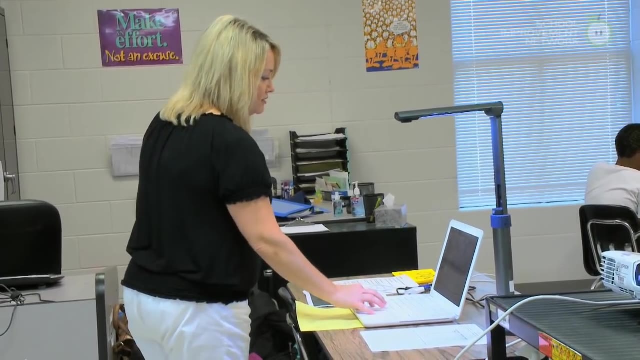 Probably not. Probably not, but we could get close using the data that we've already collected. right, Okay, I want you now to predict. Let me ask one more question: Does it matter if I used 0,12, and 0,7?? 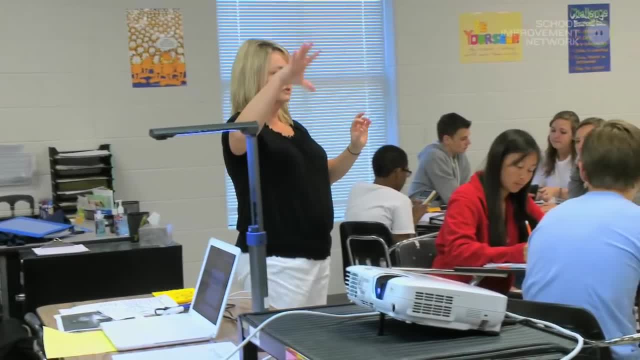 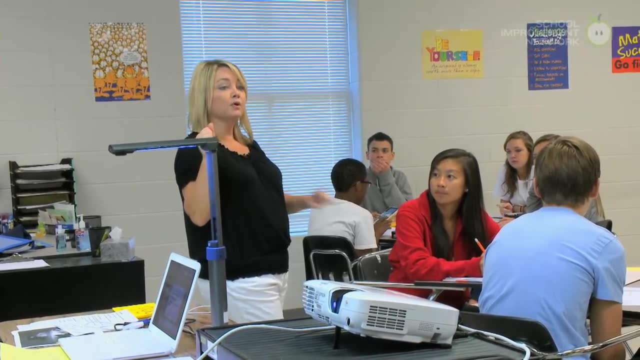 0,, 12,, 24,, 36, or 1900,, 1912,, 1924, does it matter? with my, will it change my prediction? Well, not change your prediction. but what will be different? Your equation will be different. 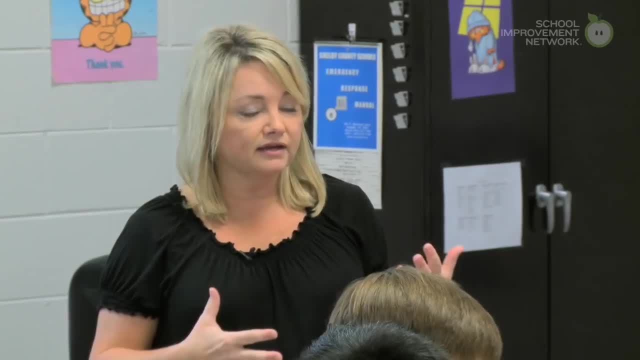 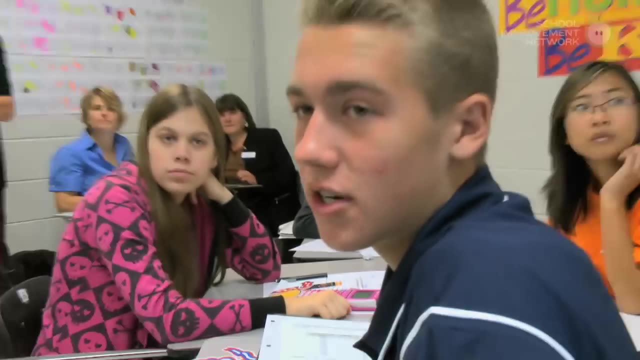 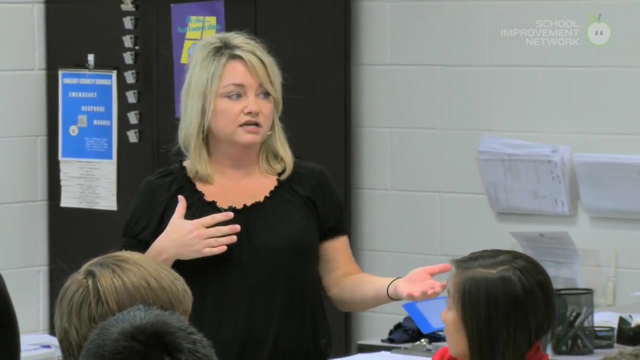 Your prediction equation will be different, but that's okay. If you use 1900s, what kind of year are you going to enter for your X? The exact year that you give us. Perfect, Okay, If I started at year 0, am I going to use the exact year? 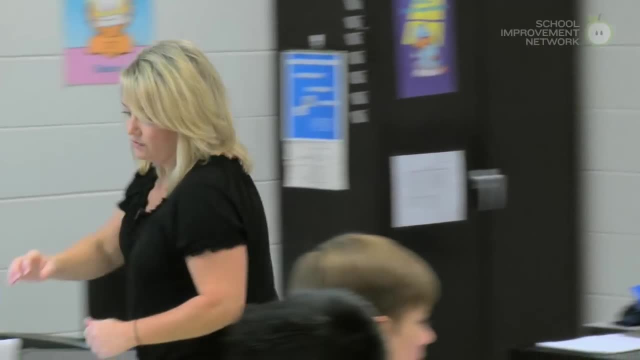 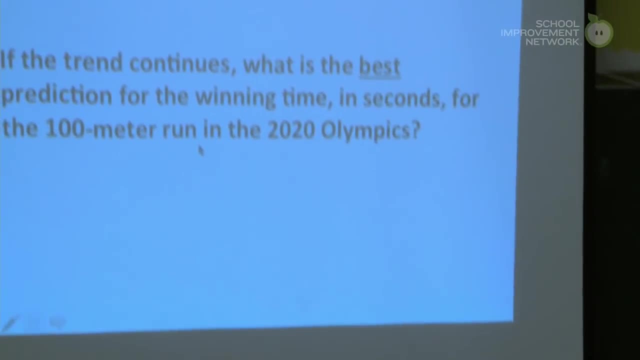 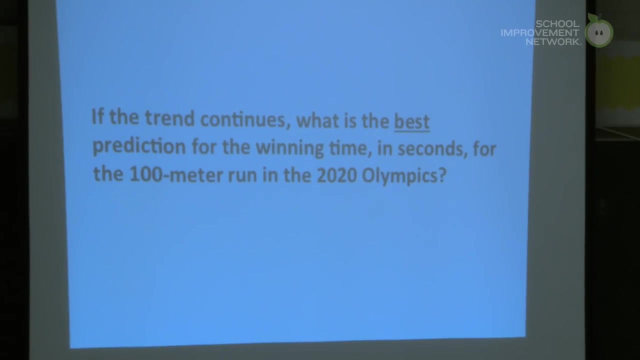 No, No, You're going to correlate that. Okay, Let's try one. I want you to predict the winning time for the 100-meter dash in 2020.. Okay, Predict the time for the winning time for the gold medal in 2020.. 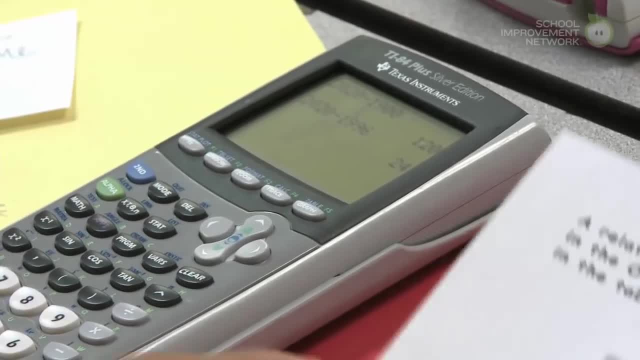 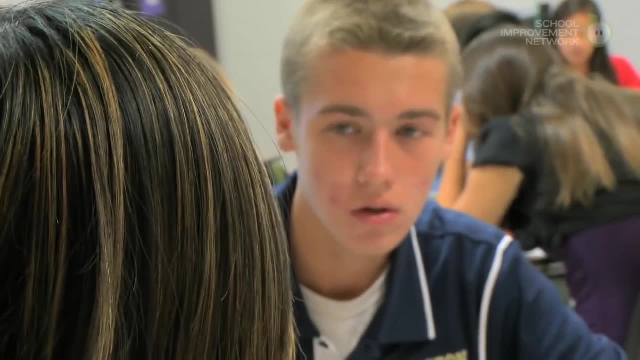 That's why you didn't have that. Thank you, You're welcome. Are you rounding? She gave us 2020.. X is 2020.. So you do, Y equals A plus B. So what are you going to use for your X? 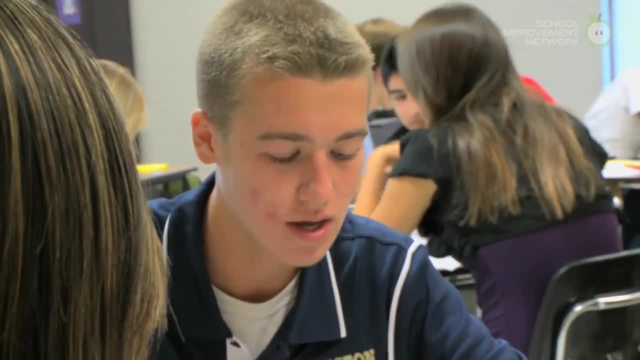 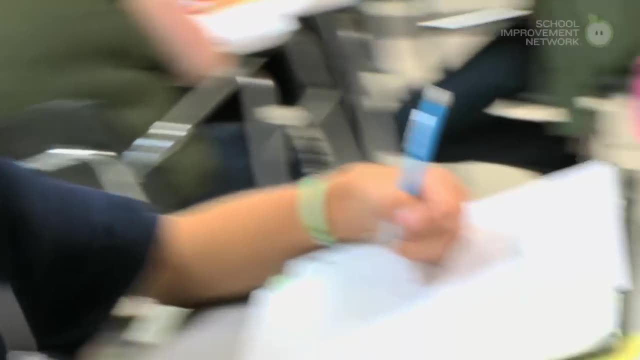 A is 32.. No, A plus B times X, That's A You have to have. is that exact? Well, nothing can be exact, I know. but is that like the decimal? like no rounding, I rounded it. 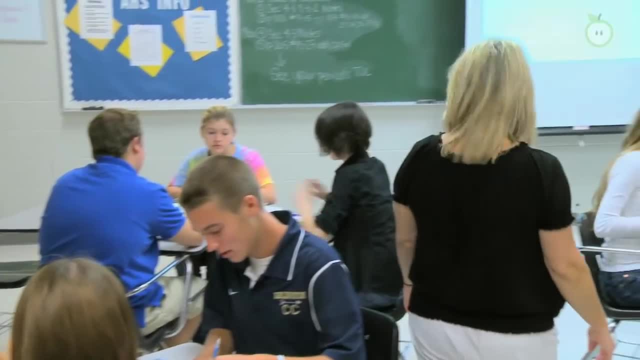 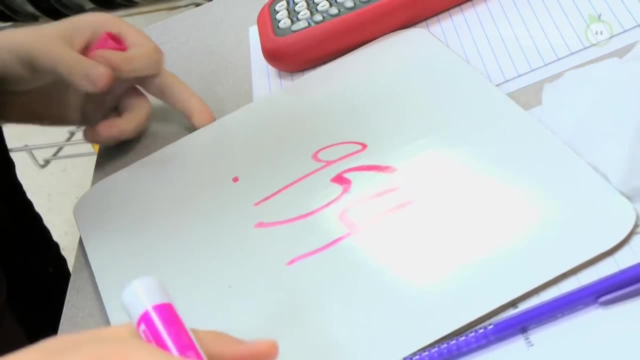 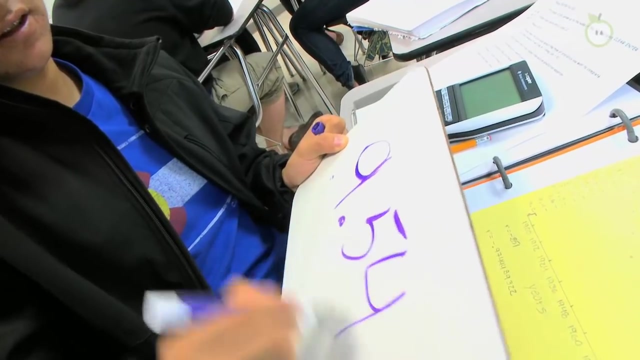 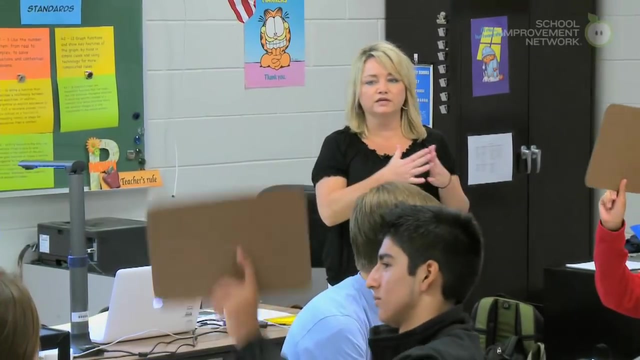 What would you do? All right, Write your answers on your whiteboards when you're ready. Okay, Can you round? Okay, And did you what? did you enter your L1?? Okay, Let me see those whiteboards. What's your prediction in 2020?? 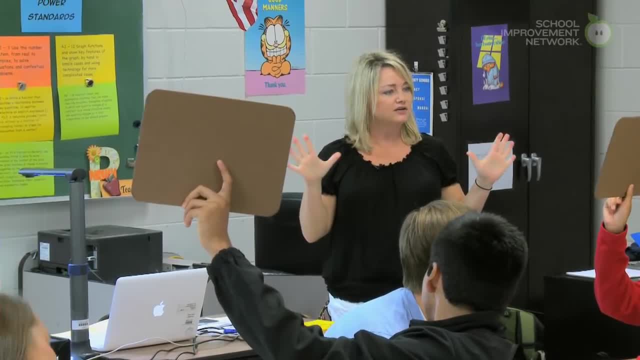 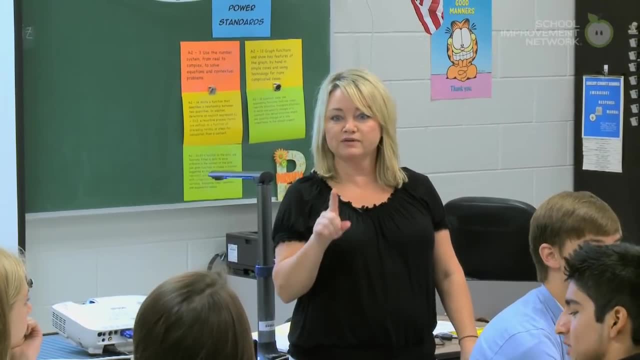 Yay, 9.54 seconds. Everybody got it. Awesome, Awesome, Okay, Did anybody watch the 100-meter dash in the Summer Olympics this summer? You did, Don't give it away. Do you know the time he ran it in? 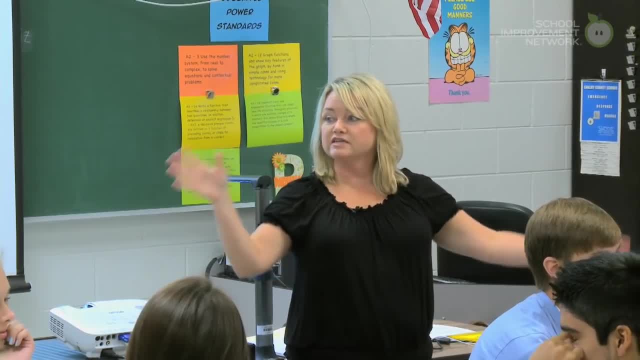 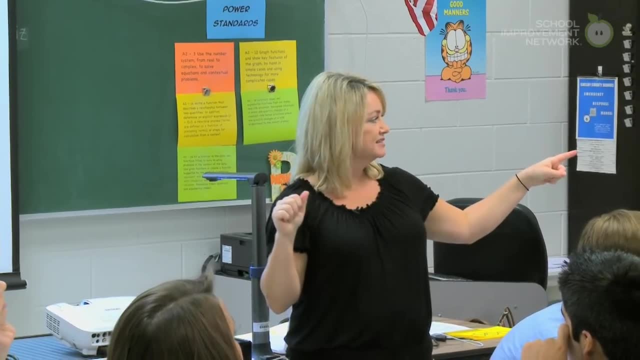 I have no idea. No idea, Okay, good, We are going to do the exact same thing, but we're going to do 2012 this time, Okay? Does anybody know who the winner was? Bolt, Bolt, Bolt's the one that ran it. 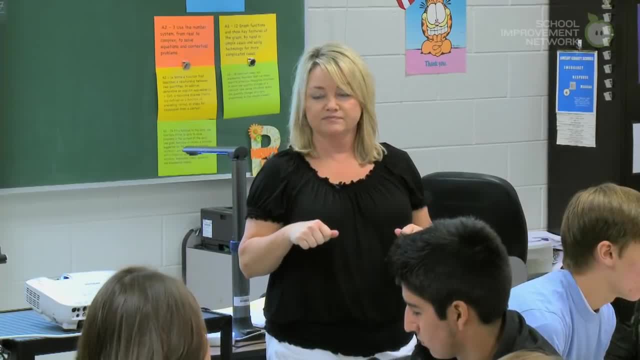 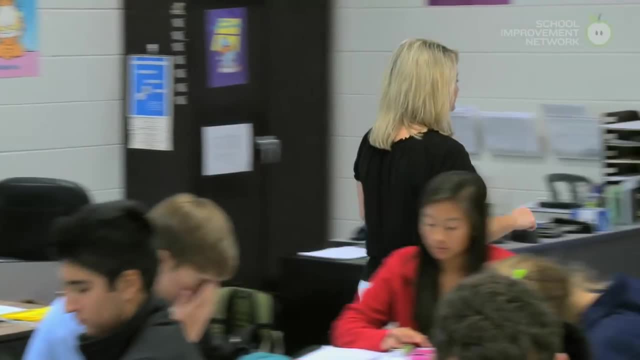 I want you to predict what he won: gold as this time. Do your prediction for what Bolt ran the 100-meter dash in at the Olympics this summer. Not yet, Not yet. Let everybody do it. When you get it, put it on your whiteboard. 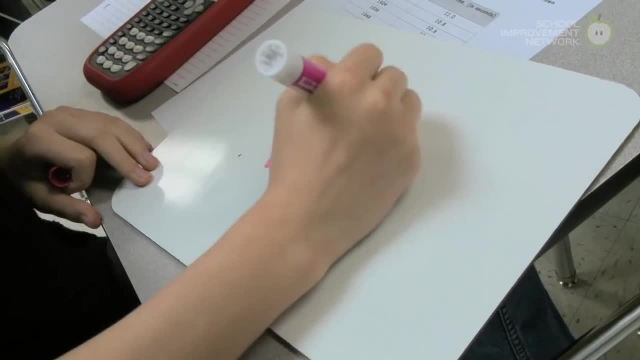 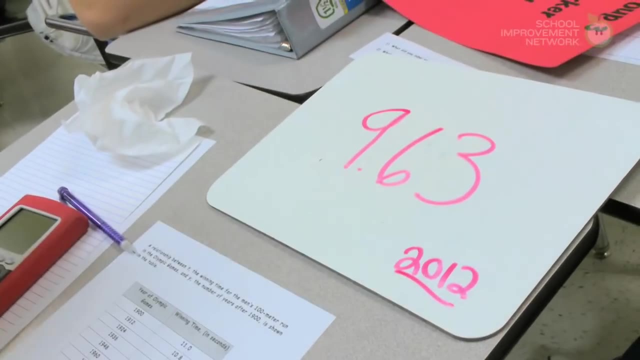 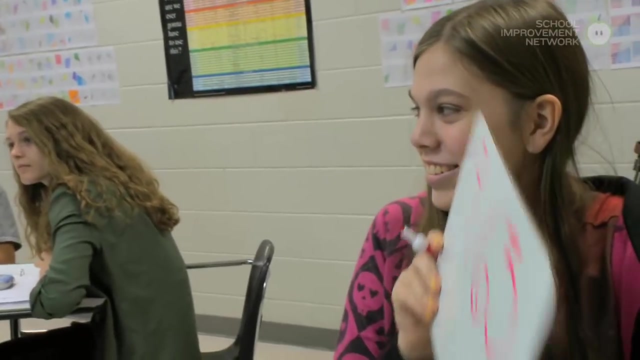 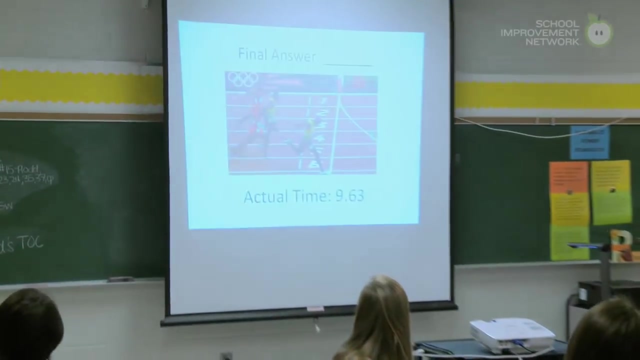 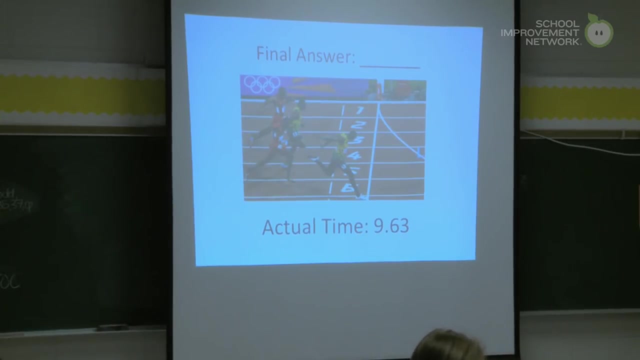 And round to the 100s, Hold up your boards. Can anybody do a drum roll? because I can't. Awesome, Ready, That's weird. Yay, whoa, exact, exact, isn't that cool, kind of neat. okay, i want to talk about our data and the future. 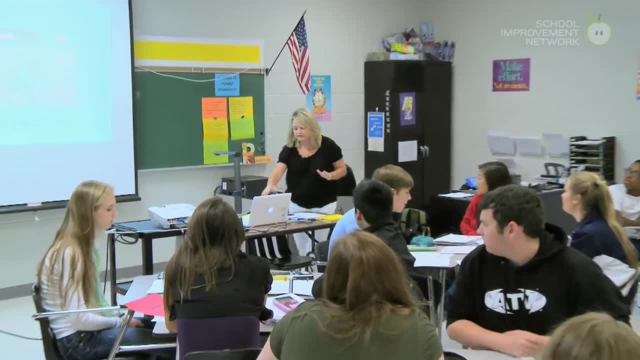 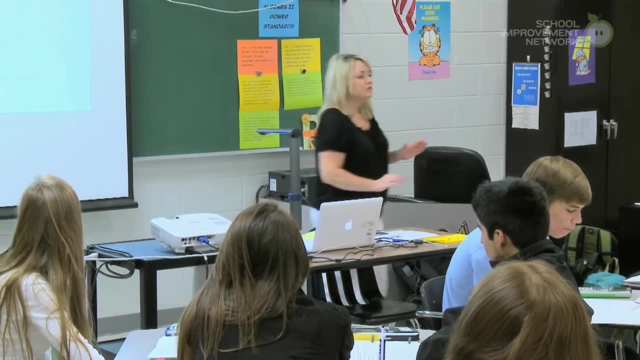 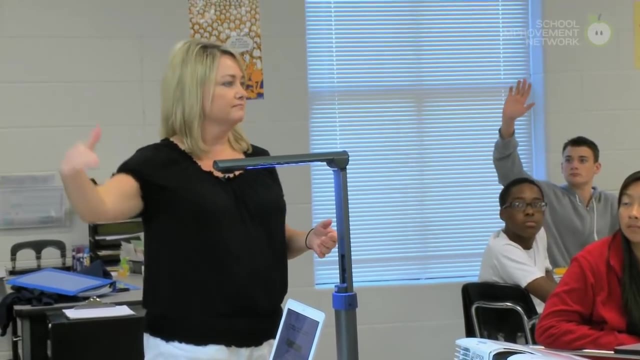 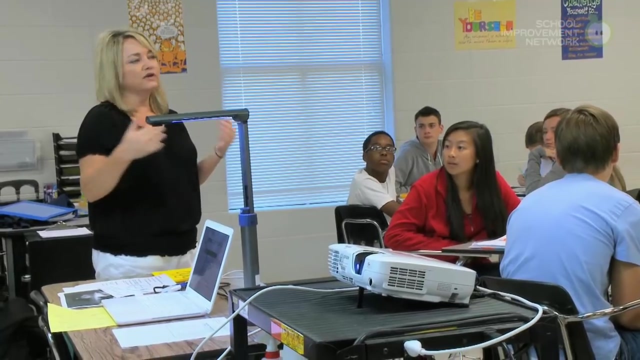 okay, now your original data. if we go back and look at that- your original problem, right? what's the trend? starting at 1900 to 1996 and even going to 2012.. what's happening to your winning time? it's decreasing right. so it's going down. so i want you to think for a second. how long that? 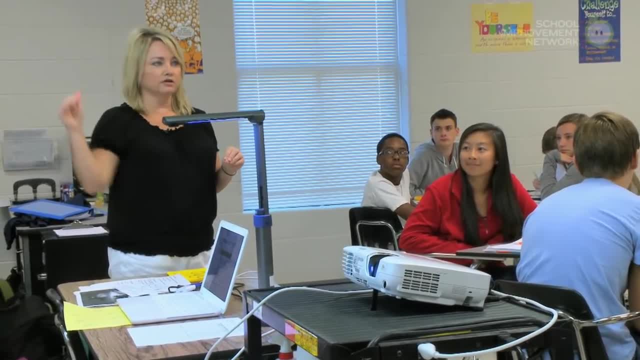 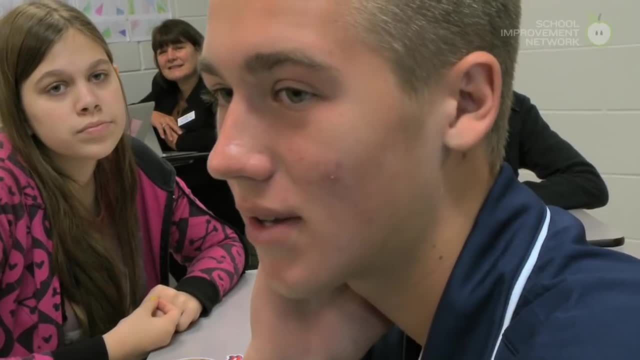 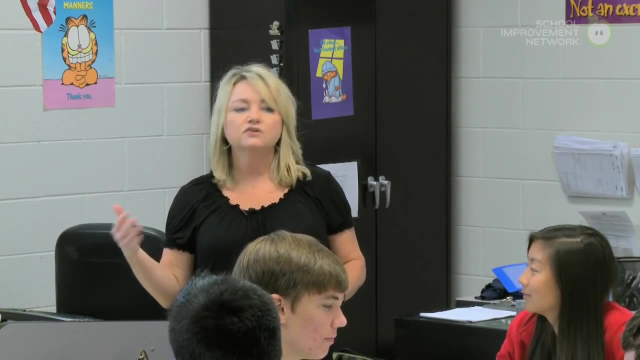 trend could continue. could it keep decreasing and decreasing and decreasing, thomas? it might keep going down, but eventually there might be such a good time that's really hard to beat exactly. could anybody ever run the 100 meter dash in zero seconds? no, so eventually what's? 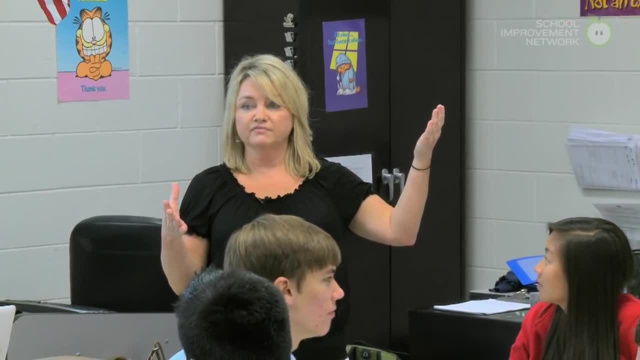 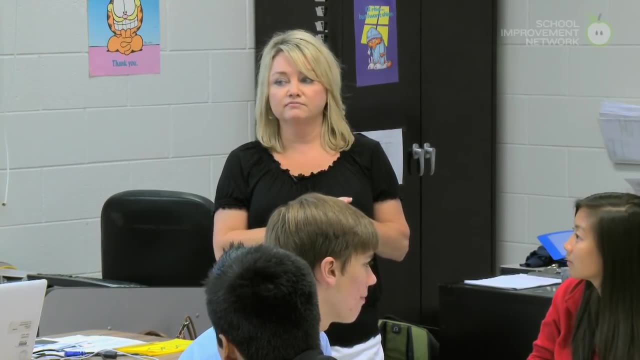 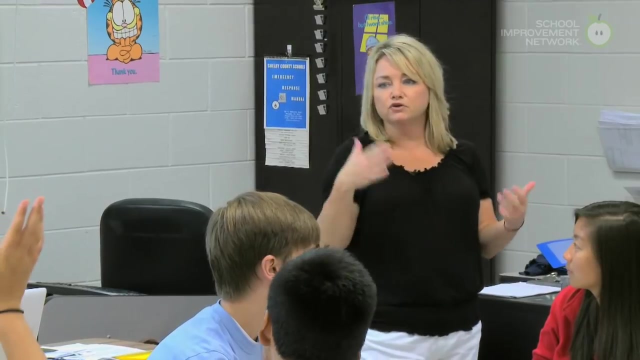 going to happen to your graph. it's going to level out, it's going to go horizontal. would that change your correlation coefficient? yes, it would. okay, let's think for a second about who could use this data, who could use information like that. what kind of career amanda? people who are running against him? 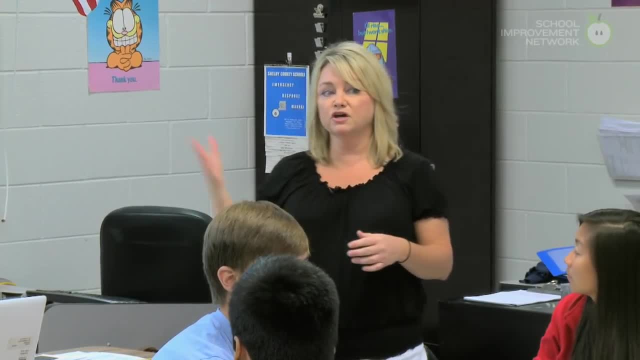 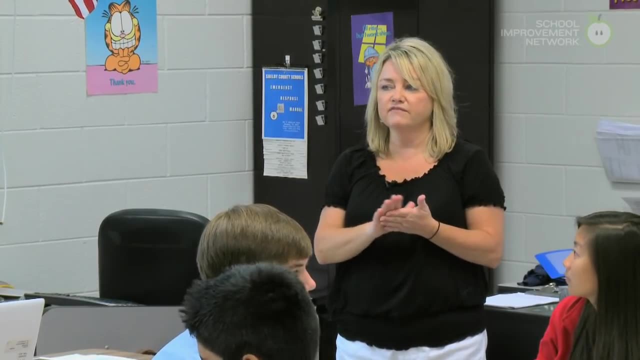 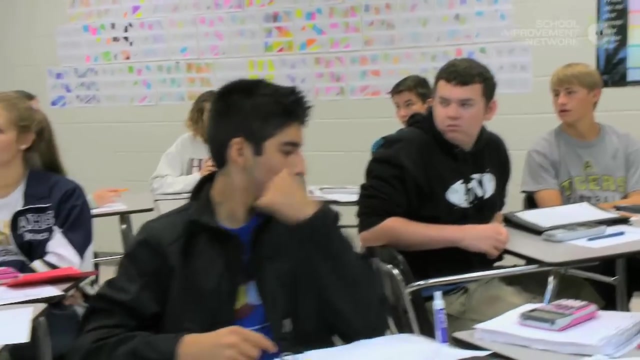 people who are running against him. if you're going to prepare for the olympics, you need to know how fast he's running. you need to know the trend of how fast people are running somebody else think of, think of other careers, other people who might be involved. donnie vegas, gambling say that. 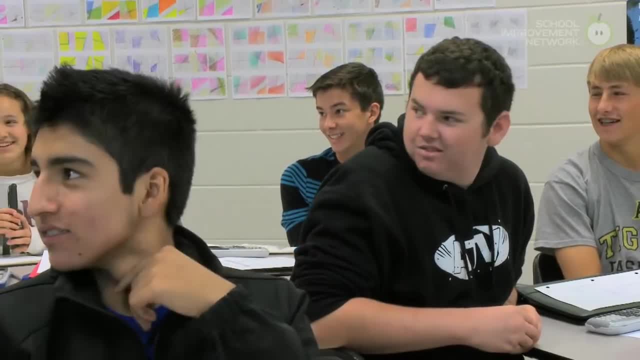 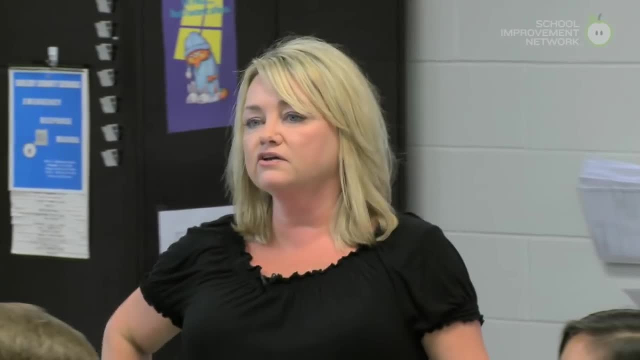 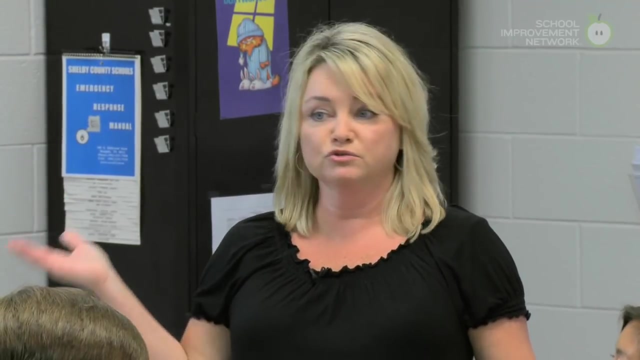 again. vegas gambling, vegas gambling. you need to know the odds. you got to know the odds. what about? um? think of a shoe company. could they use it, like nike? oh yeah, yeah. what could they do with it? they could name a shoe brand after the time. they could name a shoe brand after the time. 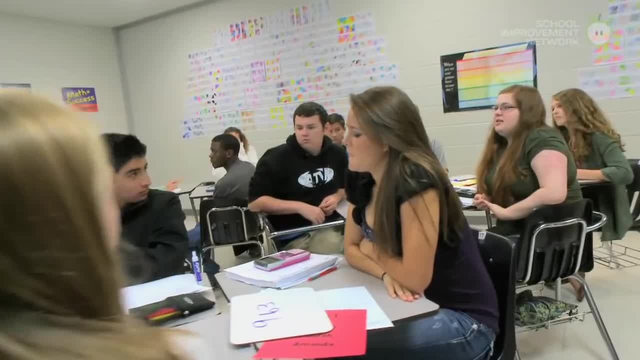 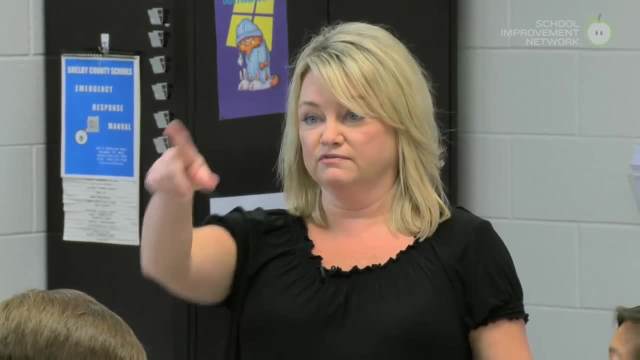 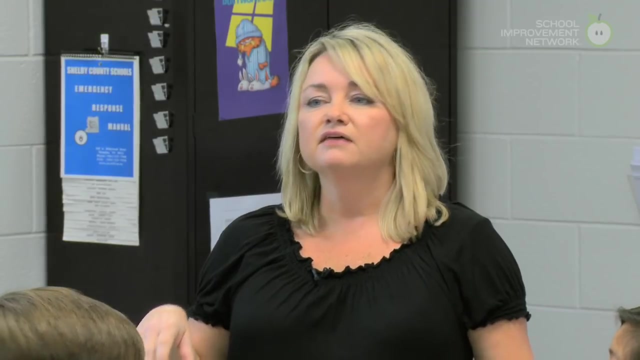 think about. maybe shelby try to create different types of shoes that are fit for that kind of speed. perfect, they could come up with a brand new shoe- kelsey people writing an article for the newspaper about it- perfect, absolutely, what about? what about if you're a commentator for the olympics and the 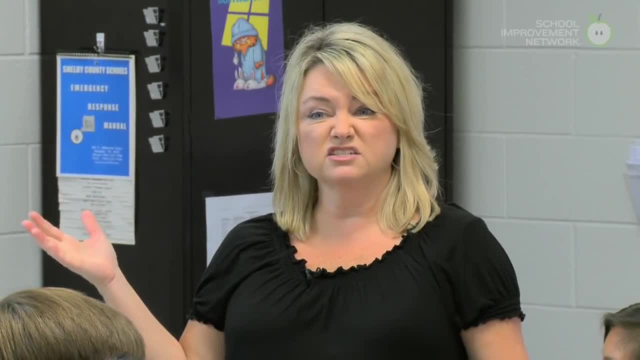 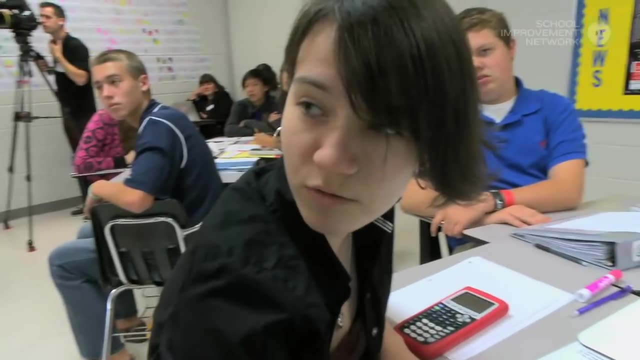 race hasn't happened yet, would it be nice to know what he might run it in. you could use that to protect it, right, bridget um? people who are investing in him will want to know if he's going to do as good as he's producing. if they're going to be in the ring, it's really voorstelling to know. 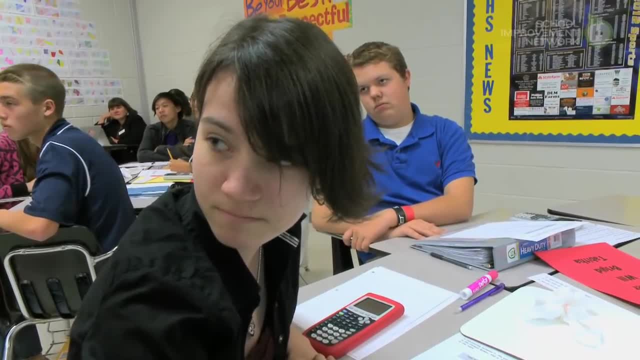 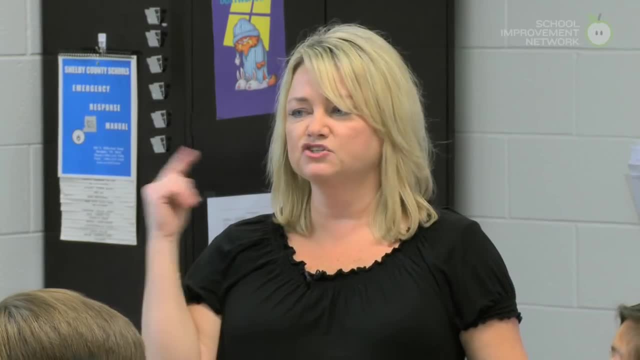 if he's going to be in the ring. if he's going to be in the ring, i think, i think it's all about him projected to, or if he's going off of his game. excellent answer, very, very good. what about the health field? okay, did anybody by any chance think performance? 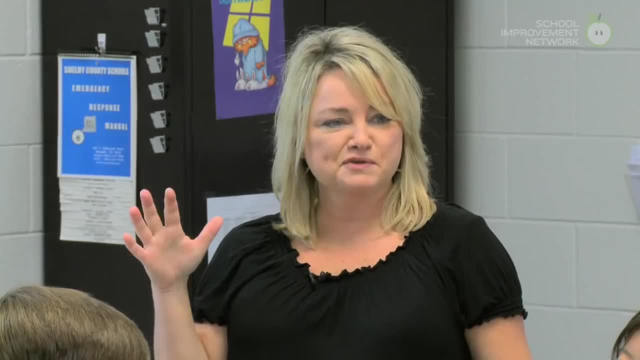 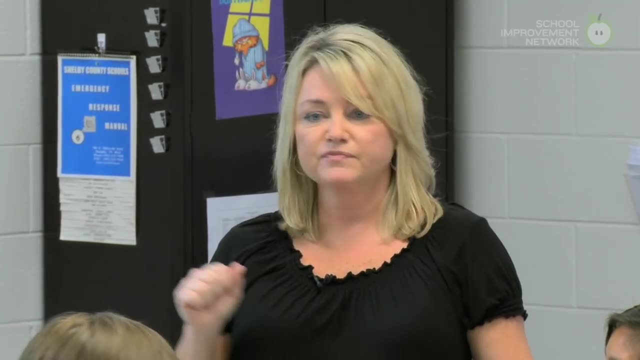 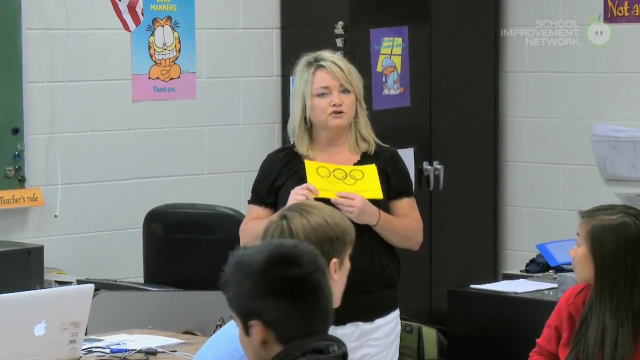 enhancing drugs or anything like that. yeah, a little bit, but even for the better, for health. okay, you could even in the health field. maybe they could use this data. okay, all right, we're gonna do one more thing. this is your exit ticket to leave the class today. okay, and this is by yourself, not in your group. I want 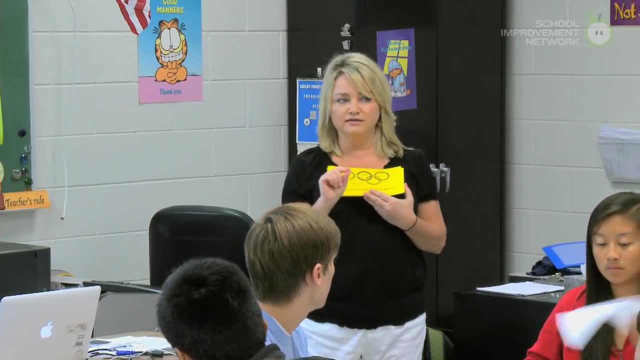 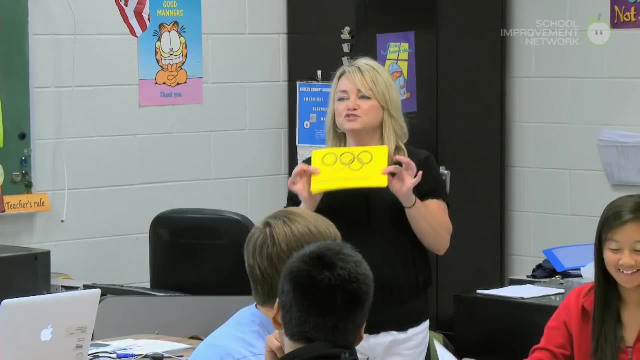 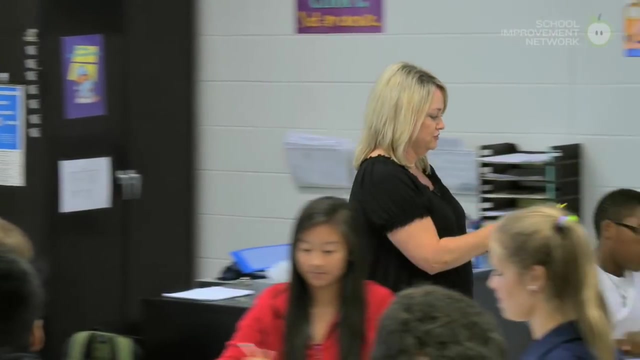 you to predict what you would have to run the 100 meter dash in and girls just pretend like you're running in the men's final. okay, what you would have to run in 2016 to win gold. okay, and explain your answer to me, what time you would have to.